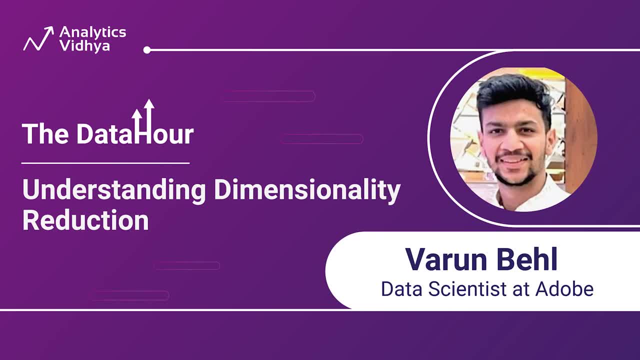 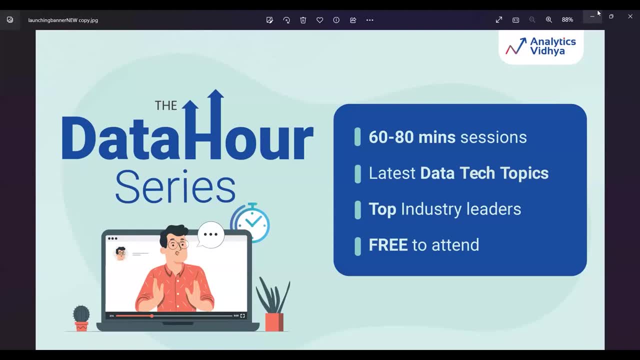 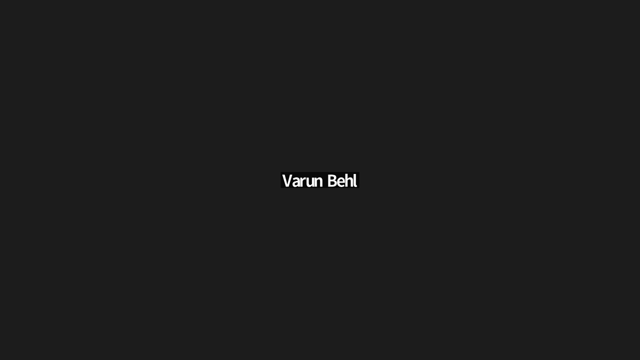 Welcome all to the second part of the data series session. second part of, actually, my data series session, where initially we had discussed around understanding the concepts of the data. However, in this session we'll be continuing that particular series only and talking more about data, and we'll be covering aspects of dimensionality reduction, which 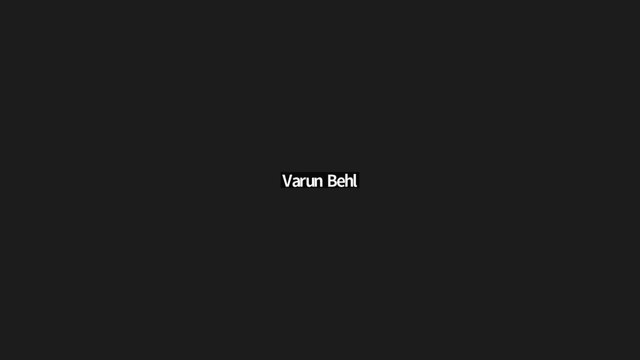 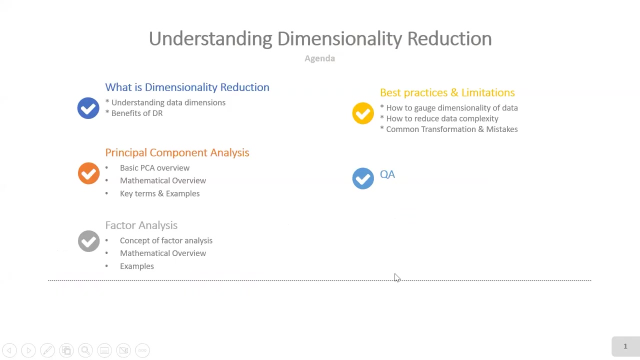 is again an important aspect that you have to consider when you're transforming your data for any machine learning use case. I will be presenting my screen, So the agenda for today's session around dimensionality reduction is understanding what dimensionality reduction means. what is actually a data dimension? how do you interpret data dimension does? 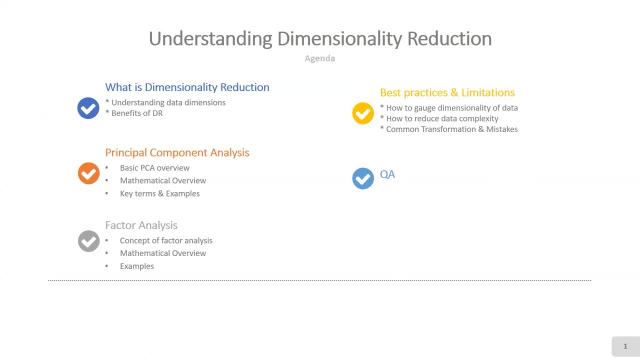 it, tell us anything about the dimensionality reduction and how do you interpret data dimension? And then talking about what are the benefits, although there are as well limitations to that also, but that we'll cover when we are talking deep into principal component analysis. 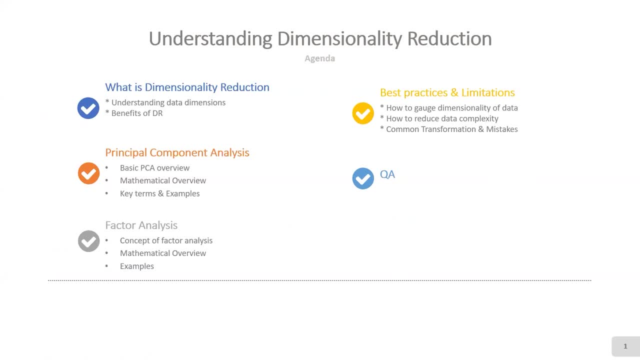 and factor analysis. So I'm covering these two aspects majorly because these are the two most used techniques and the most sophisticated techniques when we talk about dimensionality reduction. PCA and factor analysis are most widely used when you have to reduce your data and you don't have to deal with dimensionality reduction. So I'm going to talk about the 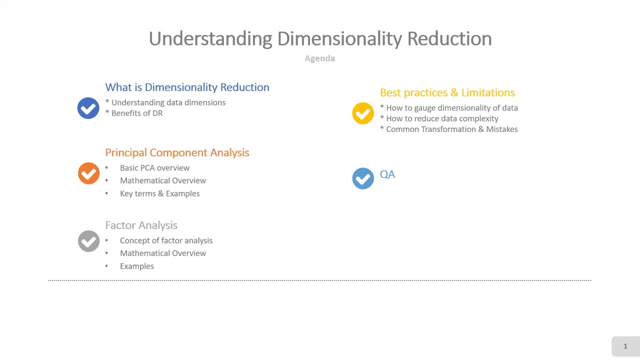 multiple lines of code and multiple algorithms that you need to create on your end. So this is a predefined algorithm that is available out there. It is there in multiple Python and R libraries, So it's freely available and it is easy to interpret as well There. 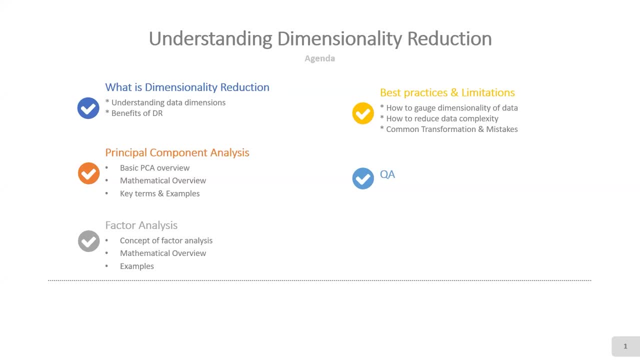 are some niche limitations to it that we will be discussing in this session. There are certain best practices that I also want to cover around, based on the experience that I have gathered and the best use cases that I have dealt with in theナ dungeon. Lets get into detail. So the best practices that I would like to cover in this session. 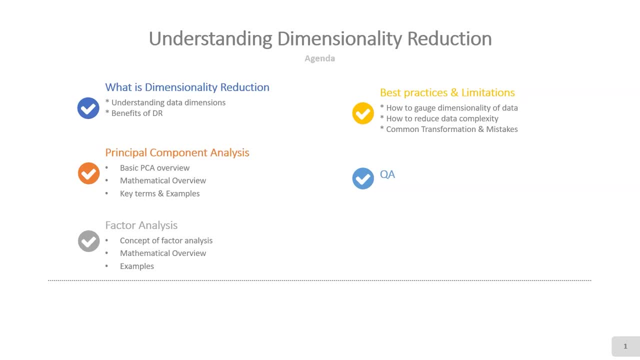 are the following. the first is to know if everything is in perspective or contemplative, One which will help you in understanding these two algorithms better and not make the mistakes that generally people do while handling these algorithms, And we can have a brief Q&A if time permits. 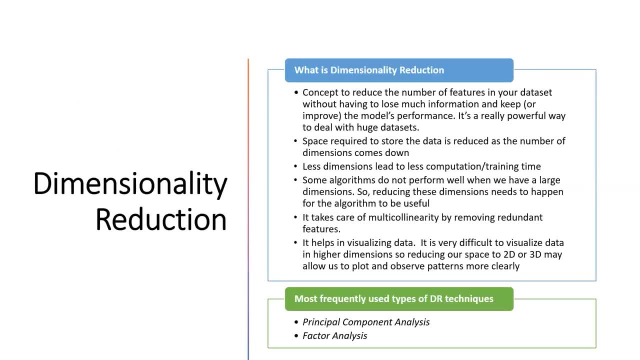 So yeah, moving into the session talking about dimensionality reduction From my last session, I will take some pointers from there. Whenever we are dealing with a large chunk of data- let's say we are dealing with a web analytics data which is recorded every session, or a patient-level data- 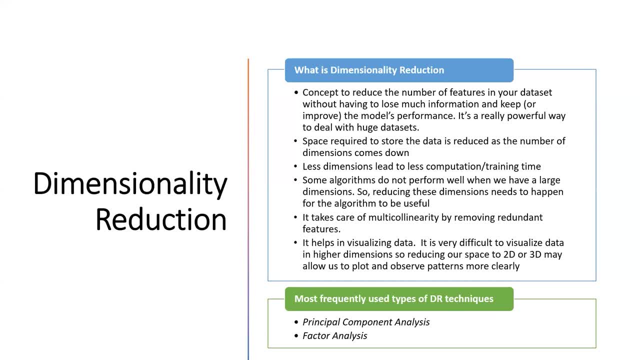 or a retail data that captures any transaction of an e-commerce website. This is a huge amount of data and primarily captured every minute that we are dealing in our day-to-day life. So to compress this data and to make it into a usable form, 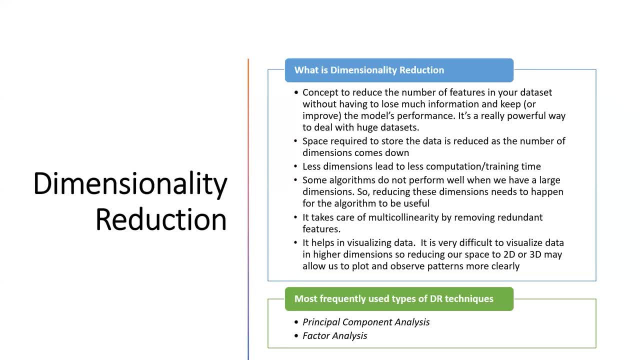 we need some kind of approach that helps us in reducing that. And then, computationally, it is easier for us to understand the data better, visualize it in a better format And even the best, The best use case is develop a better model out of it as well. 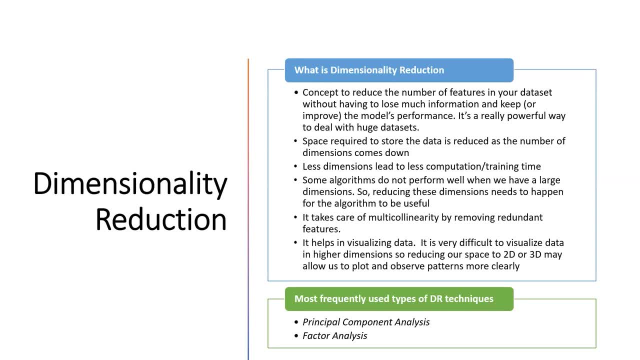 So if we look at any generic data in our day-to-day life, we have hundreds of columns. If I talk about an image data, if I transform that into a numerical format, it will have thousands of columns. Similarly, if you transform a raw textual data, 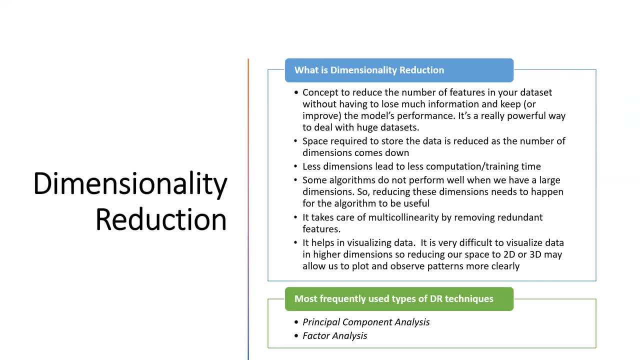 it can again have the number of. If you assume number of words as your column, then it can again have hundreds of columns there as well. So there is always a need to reduce them to a concise form, that Those concise two, three variables tell us the entire story of the data. 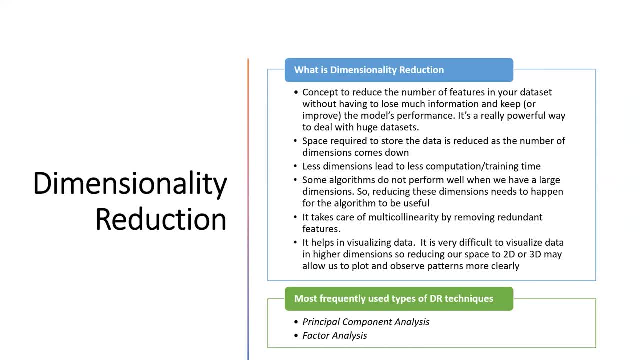 and we don't have to run our head around all these hundred or thousand columns that are there in the data. Also, it becomes easier for us to store the data as well whenever we are running any algorithms on top of that. So this is one of the major aspects that, whenever you are dealing 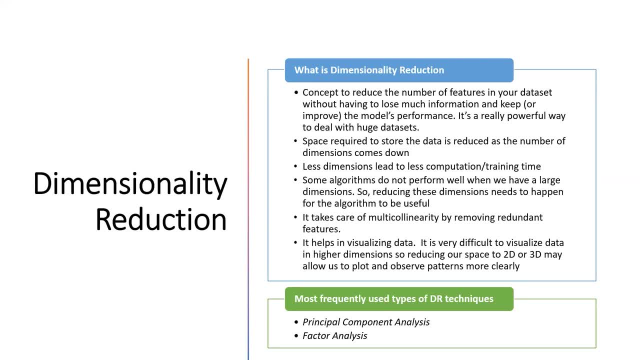 or working on your local system and people who are new to the data science field and don't have a sophisticated system at their place. it is always beneficial that you go use such approach. that helps reduce the size of the data, which, in a way, will help you use the data more holistically. 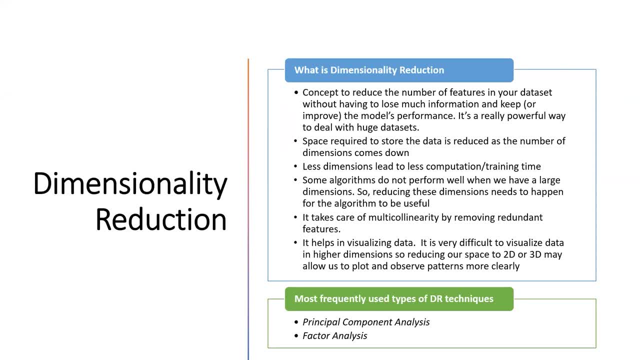 So these are certain pointers. that helps us in reducing the dimensions and as well as increasing the usability of the data. On top of that, it also takes care of the multicolonality that we usually have an assumption when we are dealing in regression scope. 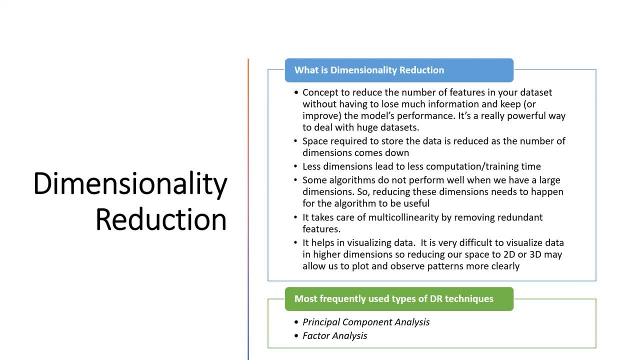 So it also takes care of these, These aspects that we usually try to take care when we are cleaning the data. So it actually takes care of all those related variables together and kind of group them together. So that's one aspect of it, And whenever you have data with thousands of columns, 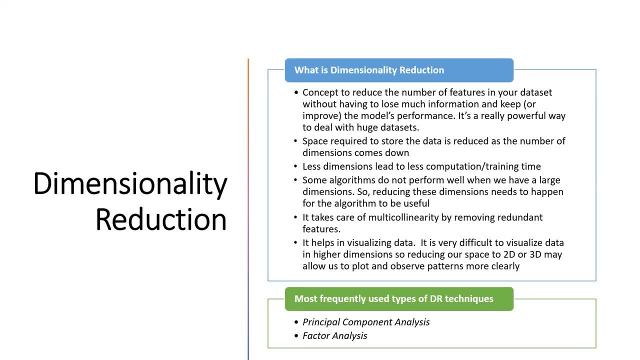 you cannot have one view of that particular data. You cannot visualize it in a 2D format. If the dimensions are even more than three, then also it's very hard to visualize any kind of data. We can actually visualize data in a 2D. 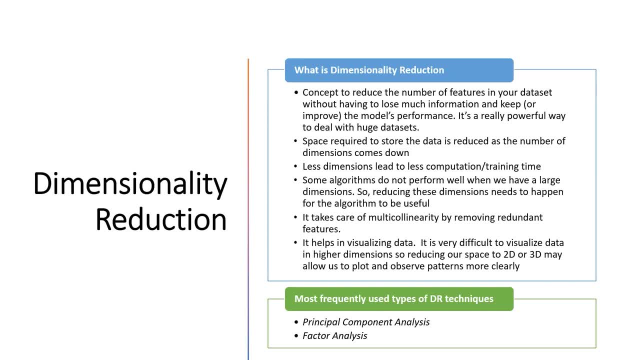 or 3D format. But when there are thousands of dimensions, it's very critical for us to know how we can reduce it so that we can visualize it in a way and make sense out of it. So, talking about the most frequently used data dimensionality direction techniques, 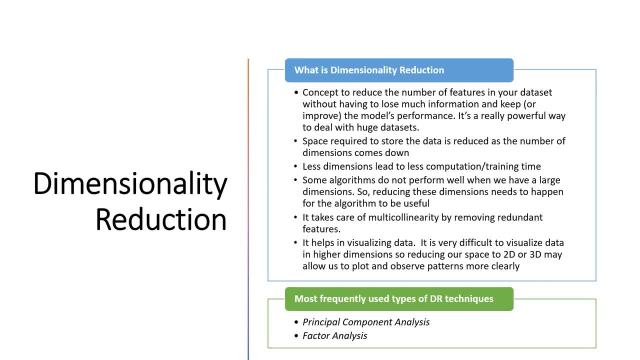 there are two major techniques that people most frequently use and are widely respected in the industry as well, because the output that they generate is much more accurate or is much more easy to understand than data. So these are some of the standard techniques that are available. 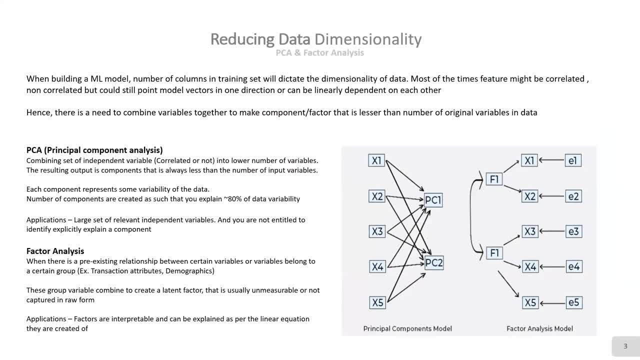 So, diving into principal component analysis, a brief overview of how these two techniques are different. We first need to understand what they actually do. So, assuming that we have a large set of independent variables in our data- and there is an aspect to this- that both these techniques are unsupervised. 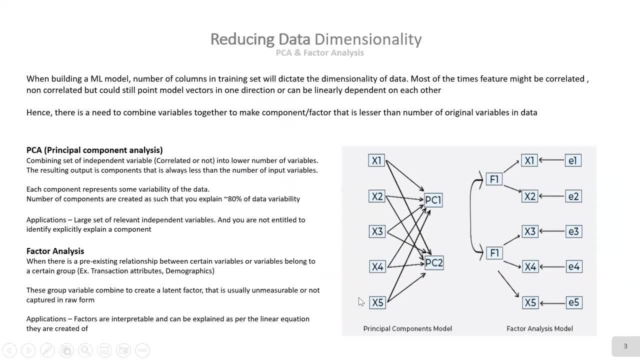 There is no dependent variable out there. So we will consider these two techniques in an unsupervised way of learning, And then what they give as an output is something like how we interpret a linear equation. So if you talk about PCA, it's like if a group of variables is reduced down to 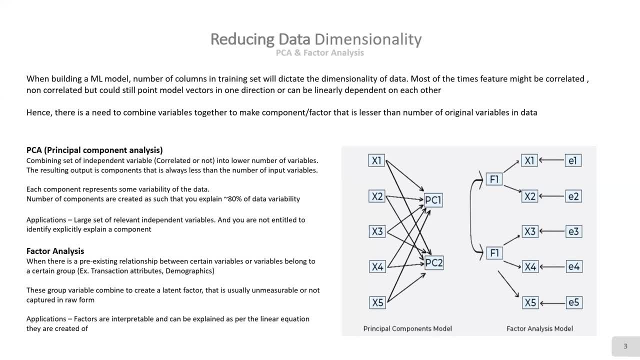 let's say there was a group of 100 variables in the data, but we reduced down to two or three variables. Doing this exercise, we are not losing any explainability or the variance of the data. The approach of PCA helps us in maintaining whatever variance was there in the data. 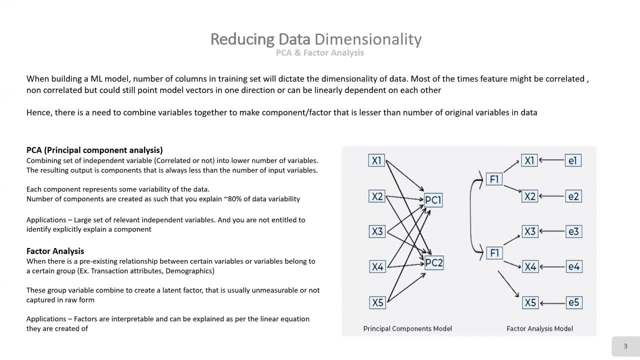 And actually holding or maintaining around 90 to 95% of that variance. So, basically, we can assume there is very less information loss, or the information loss that is even happening, which is around four to five percent. That is something that does will not have a significant impact on your output as well. 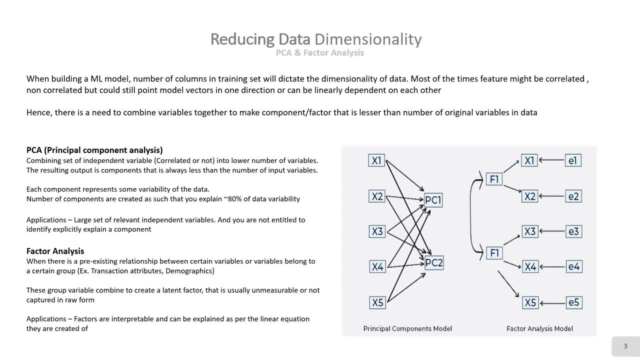 So you can assume that fairly I am dealing with the data. that was that, with the entire data that was in the original format, even after running PC or factor analysis. So first thing about PCA is, in general approach, Our independent variables are concise to a smaller format in the group of, let's say, one or two variables. 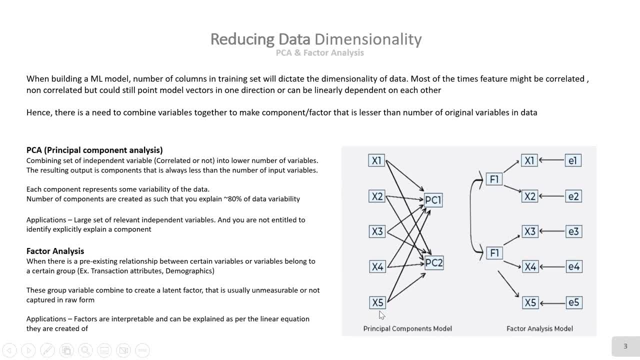 Though in PCA all the variable information will be part of the components. When I say that, I mean that PC one let's a component out of five variables, I'm creating them into two. all the value, all the data variance that is there in these five variables will be captured in one component. 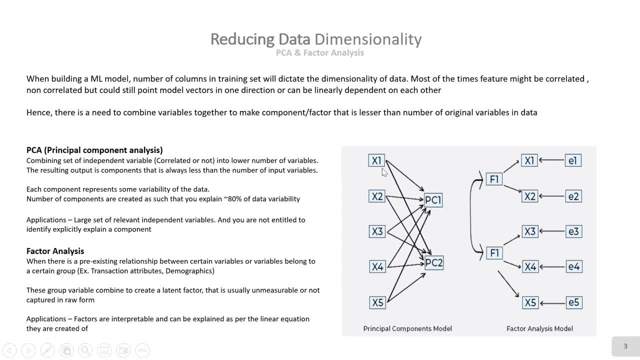 Similarly, the other component will also capture some amount of data variance, which is the value of all these factors, And one thing to note, that these are always orthogonal to each other, Like, basically, if we imagine them in a 2D space or anything. 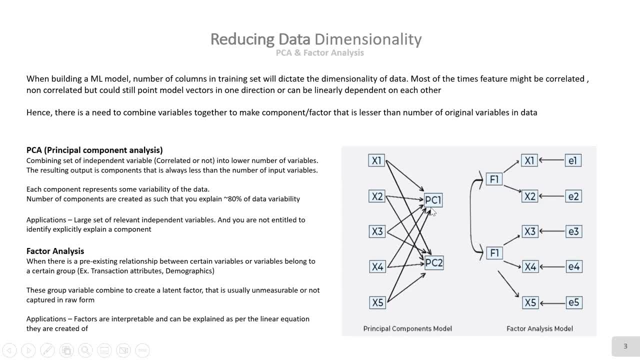 they're always perpendicular to each other. So let's say, if PC one is pointing us in X direction, PC two will always point us in Y direction, So they do not have any codependency on each other, And that is a basic assumption that we have to consider when we are building a regression model. 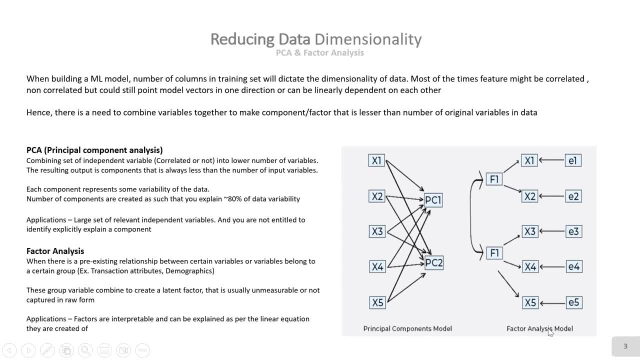 Also talking about factor analysis. Let's say we had again the group of five variables, but in factor analysis one factor would be created by a group of some variables Only. the impact of other variables on that factor would be negligible. So what it helps us is- it's a more interpretable form than PCA- that what this factor is actually signifying. 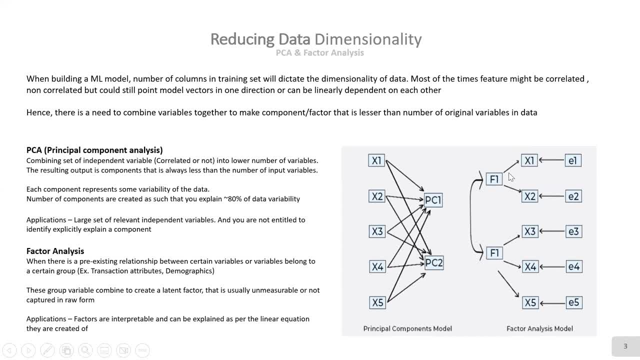 So let's say, these, these two variables were hinting at something. This variable is an inference of what these two things are combined telling you. So that's what an interpretation of factor analysis will tell you, And obviously there is some error associated. 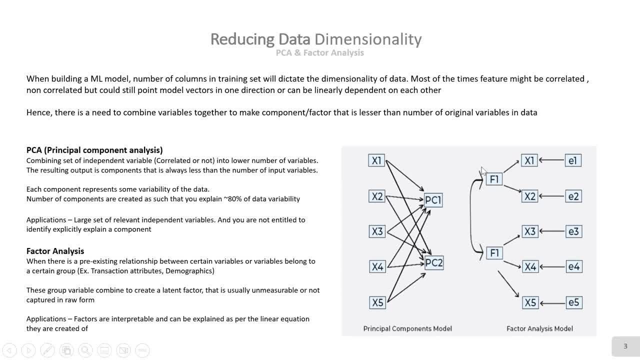 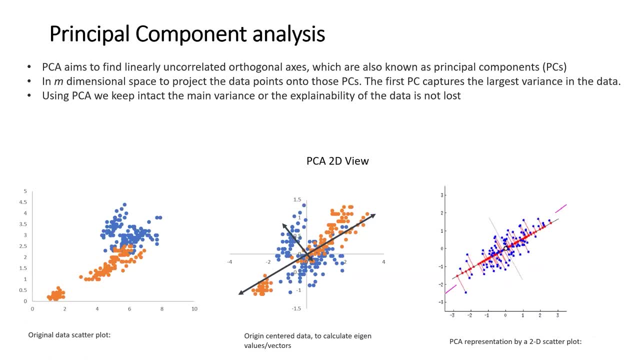 In fact, analysis that will dwell with when we go into our further slides. Now, talking more about principal component analysis, as I initially mentioned, it's a way of reducing our large set of variables into a smaller chunk. These variables could be linearly correlated to each other in the original format. 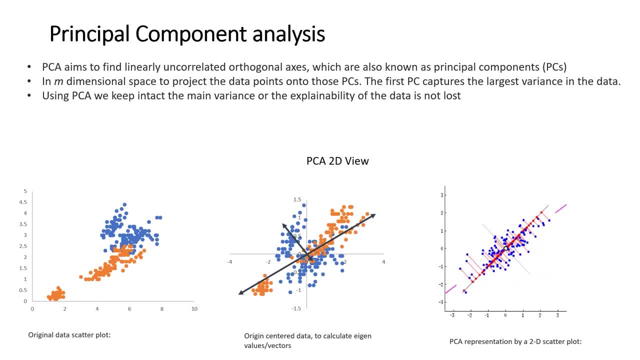 But what we get out is an orthogonal variable, variable which is perpendicularly related to each other on the axis, And there is no linear correlation between those two variables. Now, to understand how this particular thing approach, we can assume an M dimensional space of data points. 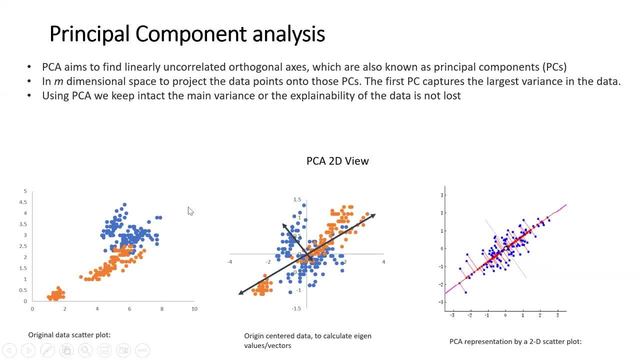 All these are scattered in a 2D space. I've, for the sake of the example, I've currently taken a 2D plot here to understand how PCA is actually working, And the main idea is that we keep intact the variance of our data, because that is the essence of our data. 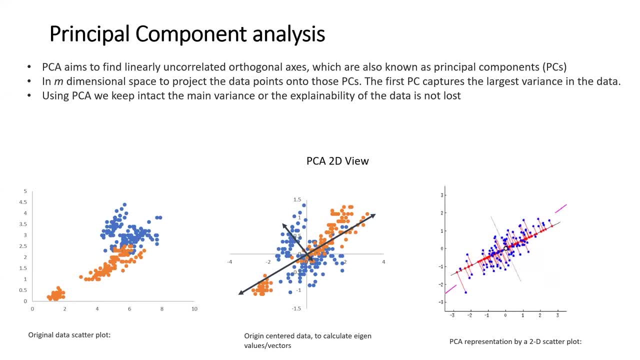 And if you are building a machine learning model, that is what's something you want to retain because, let's say, if you don't have no basic understanding of what all the fields are in your data- and there are huge set of variables- 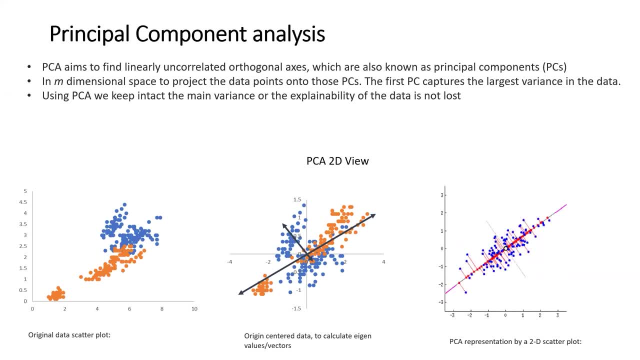 you want to drill it down to a certain extent and create a niche model, Let's say out of it, or a first draft of a model out of it. So these are the basic steps that you can use, basically having a PC on top of that, to reduce the number of columns and build a model on top of it. 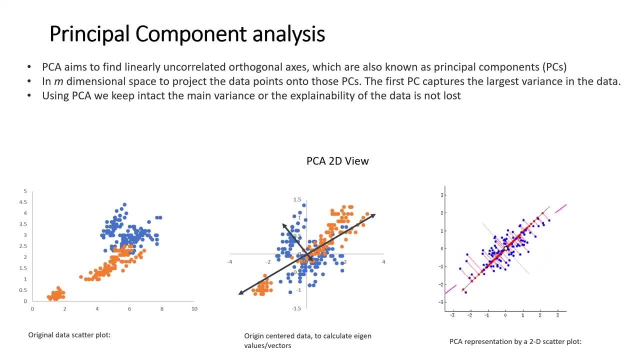 So that will keep the essence of the data as well and not help, not cause any loss of information. Let's assume I consider two categories. of how many. what was the percentage of men and women in a particular area? Now I have standardized this data to plot it on a scatter plot. 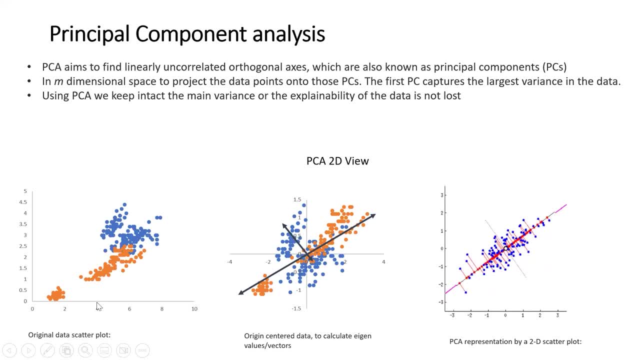 And this is across a particular region that I have captured this data. But my main hunch is that can I represent this data in terms of one equation or not? So that is the goal of PCA: that we basically create a component out of the all the columns that are there and represent it just by one component. 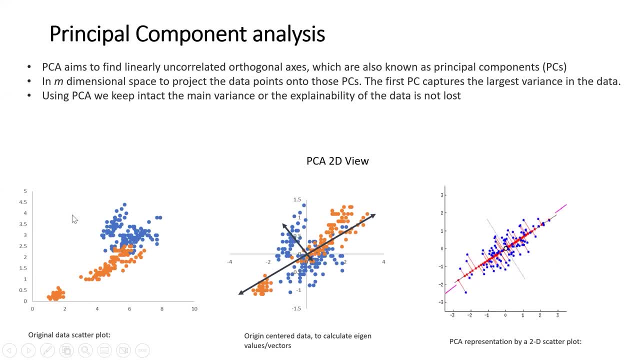 So my what, what I am doing, trying to do, is in: if you look at this particular data, it is not, it's in the, it's a raw format. These are percentages, values on both the axis is standardized, And then I have to shift this particular data to an origin center. 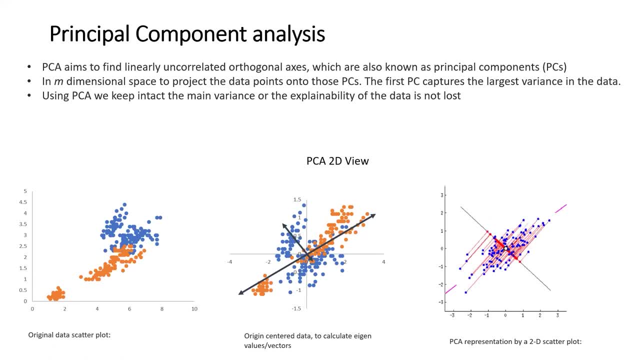 Now, this is a basic assumption when we are running a principal component analysis. that the first is we are: data should be standardized. Basically, the mean should be either zero or close to zero. Now what that helps us is that it we can plot our data in a quadrant format. 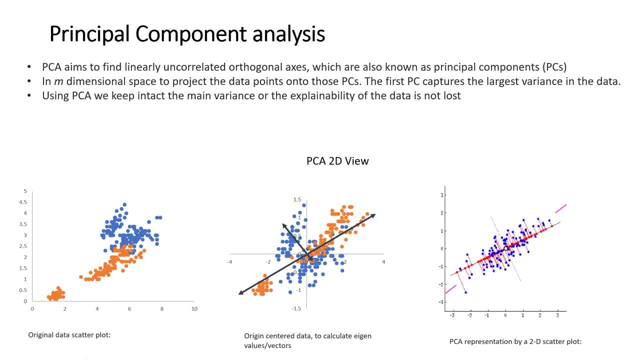 And when we do plot our data in a quadrant format, it is. it becomes much more aligned and much more clearer for a mathematical model to interpret it. Now, our basic idea would be that we are able to fit a line that caters to all these point. 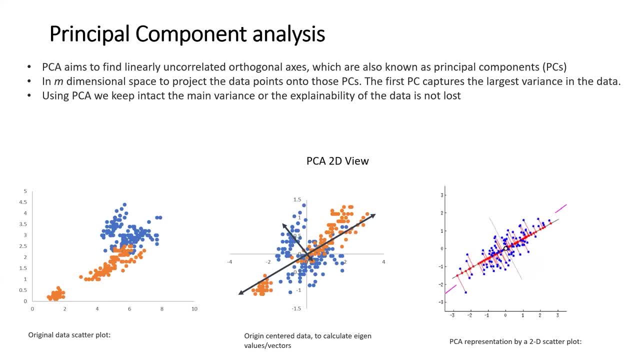 Now, when I'm saying catering to all this point, it basically is the maximum square distance from the center point. So let's say, if I'm assuming a particular point on the first second quadrant, the maximum distance that is there from the origin is when I can say my variance is maximum. explained that by that particular line? 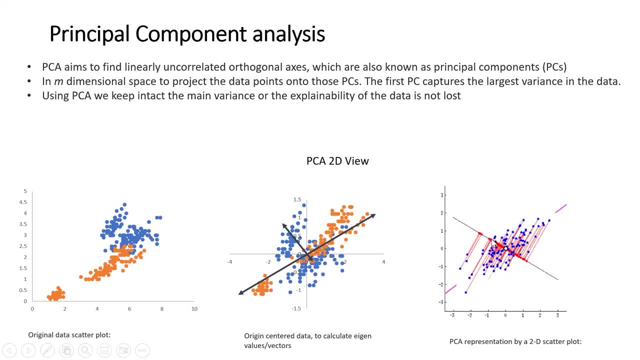 So this third image basically tells you that when we, when we are trying to get this best fit line, the model actually starts by rotation and it finally ends its rotation When it finds the best suitable point where you are able to achieve the maximum square distance for all of these points. 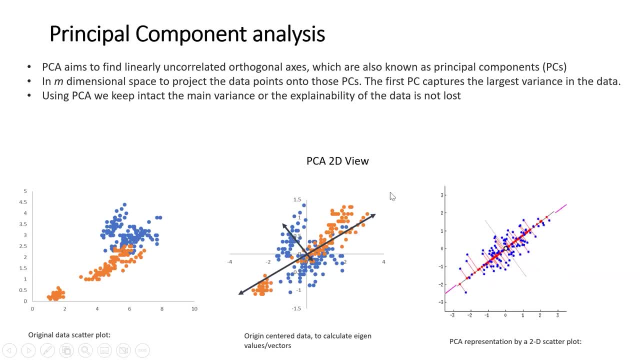 And when you are able to achieve those maximum square distance for all of these points, then we say that we have a component created. So, basically, when we say this particular line, but it holds flat, it is the point when we can say a component is created or a best fit line is there that is created. 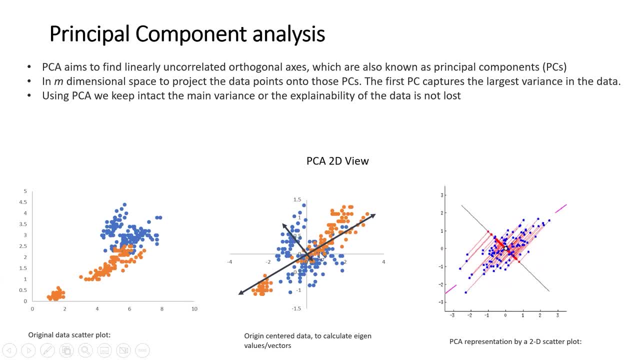 Though a singular point, like basically, as one step, the distance from this is basically, or the direction of this. basically, this of this particular line is called the vector, And this vector, in this particular scenario, mathematical interpretation, is an eigenvector. and the values of all these small, small data points that it has in it. 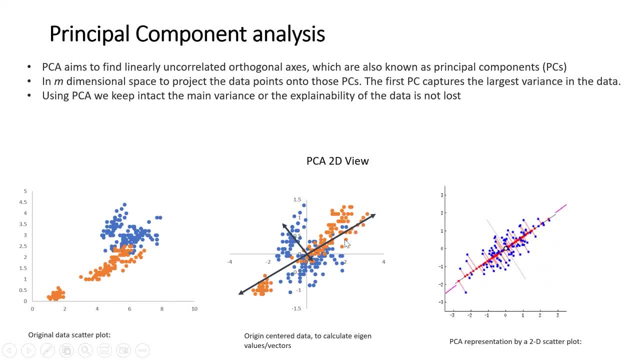 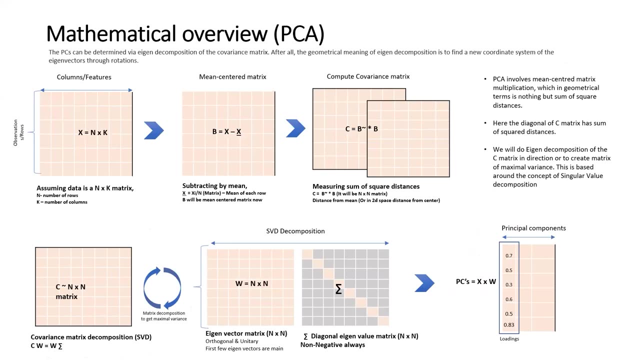 So you can assume it's a long vector and it will also have a projection or a value interpretation of all these small, small data points that are there. Those values are nothing but eigenvalues. Moving to the next slide, Now I what I was showing you till now was a very basic approach in which you have only one or three. 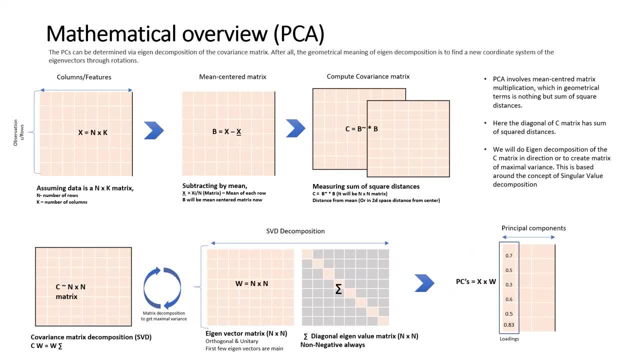 four columns in which there is one categorical column. You want to understand the interpretation, but when we are dealing with a large chunk of data, it's could be an n cross K metric, It could be any, any dimension data. It's a huge chunk of data and we always solve these kind of problems in the matrix multiplication approach. 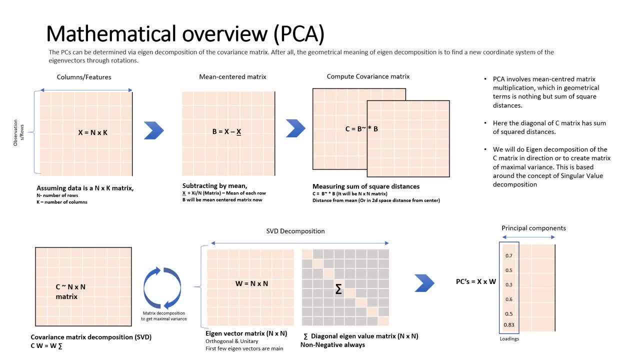 You can read about single value decomposition Also, which is the basic crux of how PC is there. I will be talking about how matrix calculation happens in PCA, and it is based around what I was talking in the previous slide, only It is how a particular vector is created. 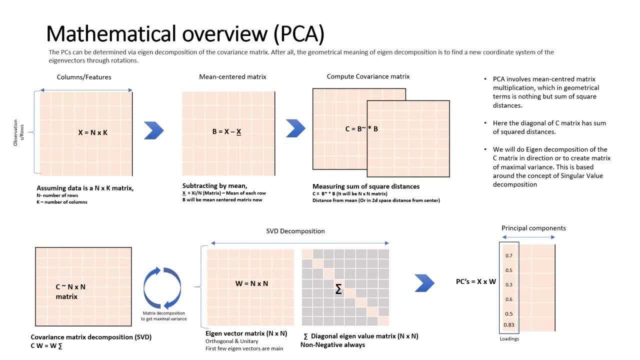 It is this the steps that we were following in that particular graphical approach. When we talk about, in the matrix approach, how it, how we can relate to that, the basic aspect of developing a component out of a set of five, six variables is that We decompose those variables. 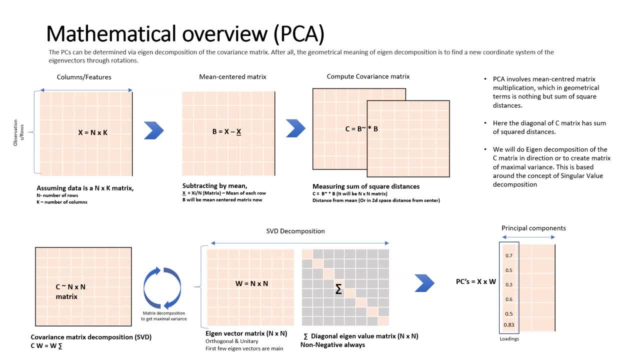 Now, decomposing variables can only be done through matrix multiplication, decoding What is the main essence of that Matrix- and only creating that Matrix output- which is important- and Kate covers all the values of the different columns- without data. So what I say here is the PCA can be determined by a can decomposition on of the covariance method. 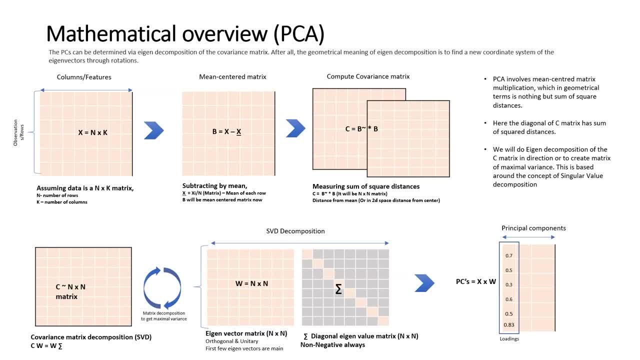 After all the geometrical meaning of Egan, this goes to find a new coordinate system of Egan vector through rotations. So, as we were seeing in previous slide, the rotation of that particular best fit line was telling us where it should stop and where the Maxima is attained. 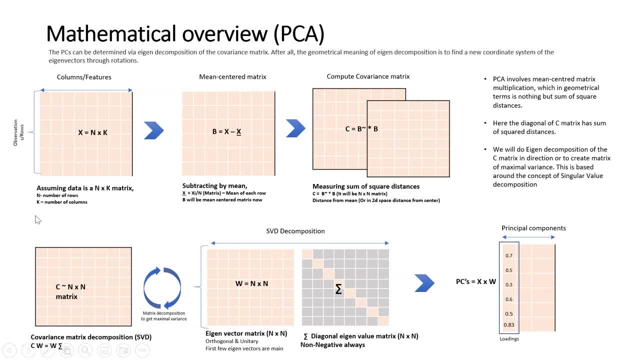 And that is the point where a component is created. Now let's assume, for an example, We have a data which is n cross K matrix, where n are your number of rows and K are your number of columns. So first, my first job is to standardize the data, or create it in the mean centralized way. 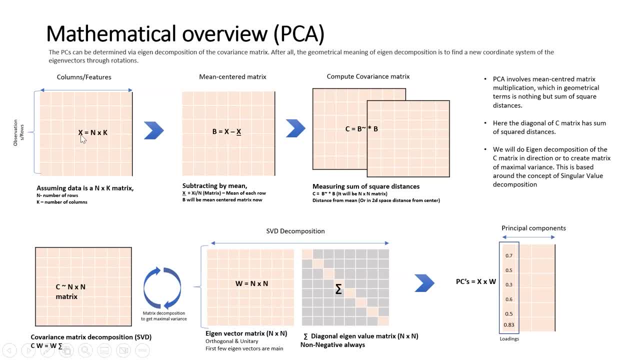 And the best way of doing that is, let's say X. I represent my data With the name of X. now, X mean X Y will X minus X Y will be a standardized format where I'm subtracting each of my value with the bead of each row. 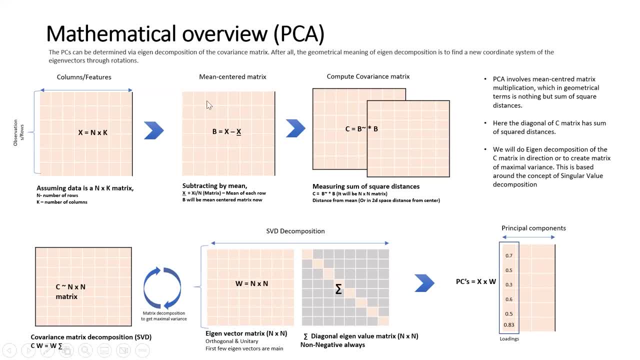 So each row- let's- if I was you- the first row- the mean of this row will be subtracted from each element of this particular thing, And then we, whatever we will have is a standardized mean, centered data. Now, when we have this, 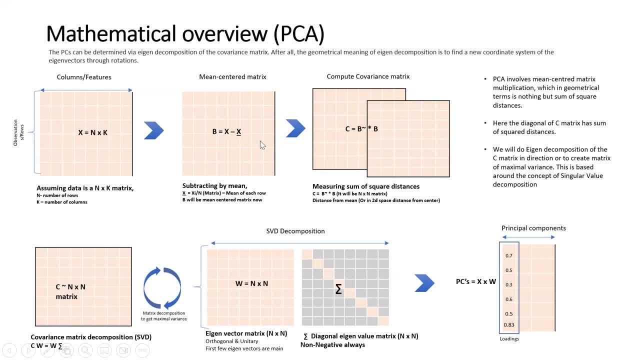 if you remember, covariance, how we understand covariance is nothing but the relation or a variance, randomness, between two variables. Now we have set of n, K number of columns. Now, when we have to understand this kind of thing, we will be multiplying each row and understanding what is the variance of the entire data. 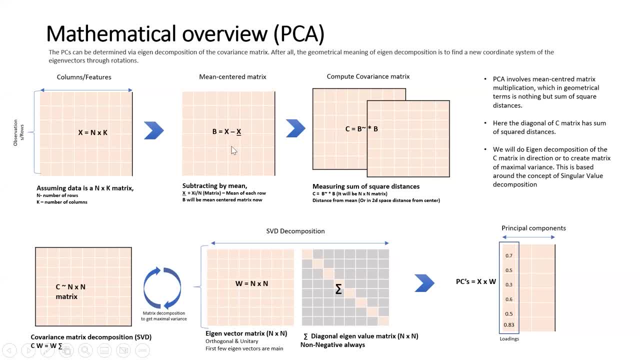 and that can only come out from a covariance matrix. So what I'm trying to do here is, let's say, B is X minus X, Y, which is nothing but the original data minus the mean of the data. I will be multiplying this data with its own transpose. 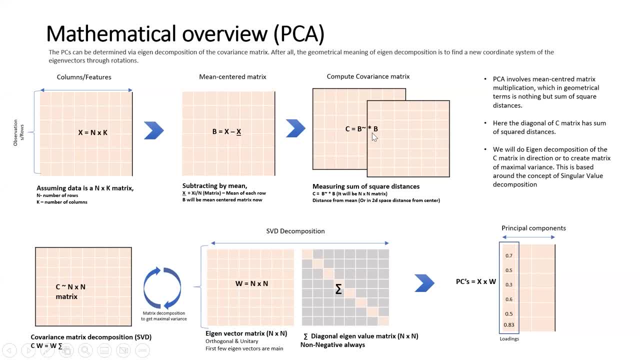 So this particular B transpose into B is nothing but creating a covariance matrix. Now, this covariance matrix will be n cross, n right, And what it actually gives me at the output is is the entire variance that the data process, like each data point in this particular matrix, or the original data, 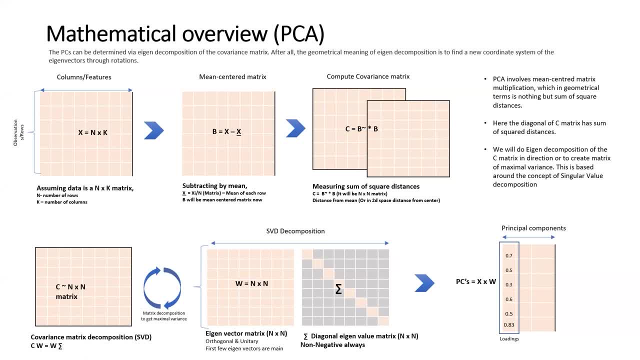 What is the entire covariance? When you have the entire covariance matrix with you, you can actually decompose into different matrices, Which will give you a gun vectors, a gun values and how the particular covariance was created. Right? So if let's say, my C variance, C covariance matrix was created here and I do an SVD decomposition, 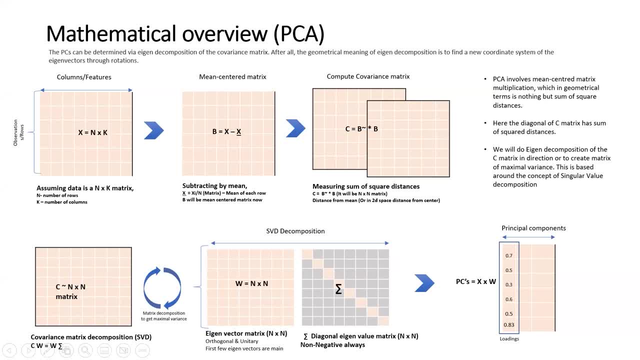 when I'm saying single value decomposition, it means creating single unitary value matrix out of a particular matrix. So I have a complete covariance matrix which has values in all of these fields. I have to Create three different matrices out of it. 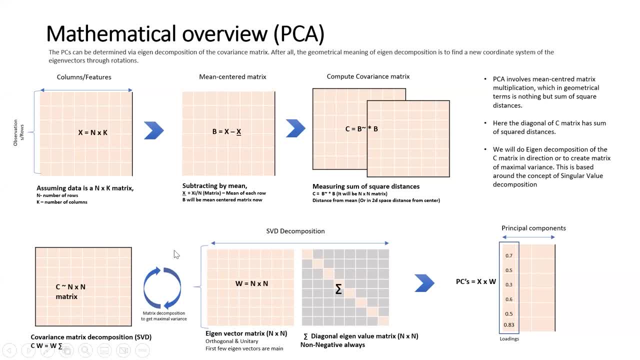 which are single value. by single value I mean most of them are of nature of unitary. Basically, when I say a matrix is unitary, it means that if you multiply it, just like how I multiplied this here with its transport, 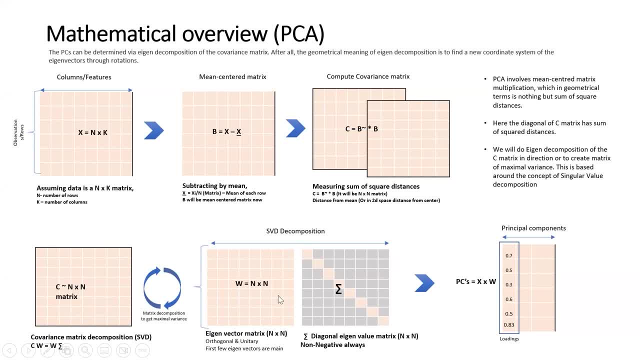 it will give you one as the output. So that is when you say the matrix is unitary, The. when I decompose these Matrix using SVD decomposition, it will give me a W? n, cross n matrix which will have a gun vectors across. 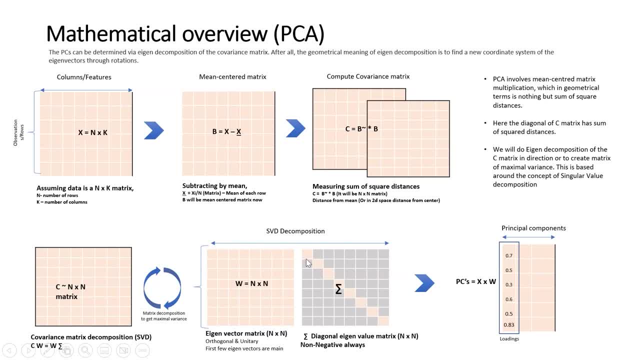 Each rows and again, it will also give me a diagonal Matrix which will possess the eigenvalues of these. Now, we don't have to use the entire Matrix. Now, what the algorithm does is it picks the only most important vectors and most important eigenvalues. 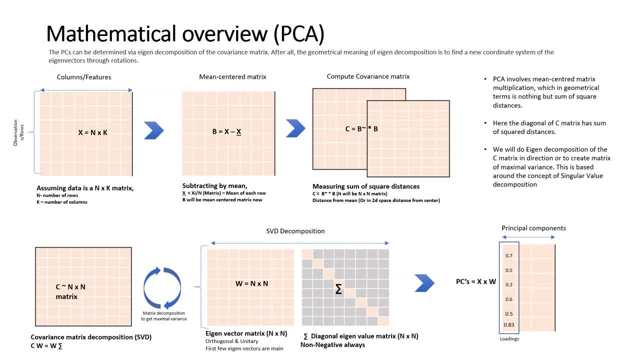 For example, the most important eigenvalues are usually greater than one, So we consider only those eigenvalues and create a data which is nothing. but I have this eigenvectors vector Matrix out. I have to multiply this with my original Data and I'll get something called a component. 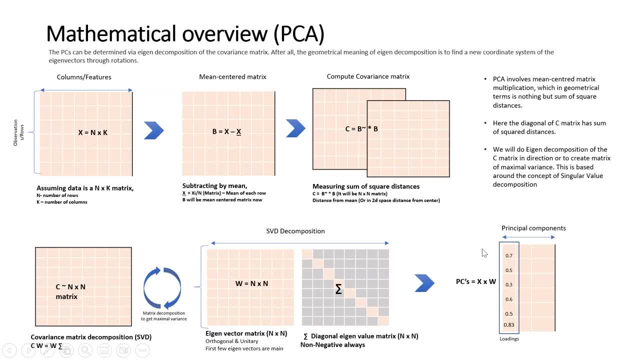 So I am picking each vector by vector and it is my, it is my, it is on me how many components I want out of it. So it is a bit complex to understand, but this is the mathematical back end of PCA. What is going behind, and it's in the Matrix format, is the most easiest way to understand. 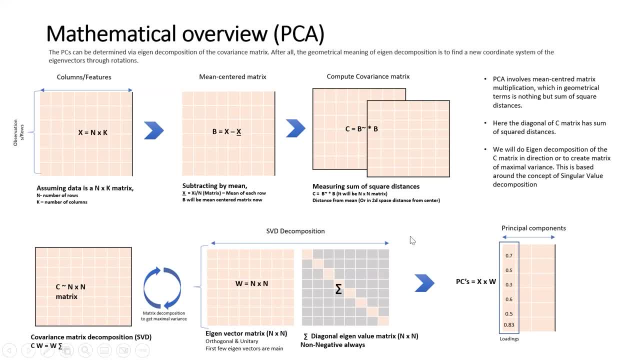 What is how the mathematical flow of PCA looks like? So, to give you a quick recap, the what we have done is we first took our original Data is standardized, or we subtracted it with our meat. Then we developed a covariance Matrix. Then we had to decompose our covariance Matrix to basically create a matrix of vectors and eigenvalues. 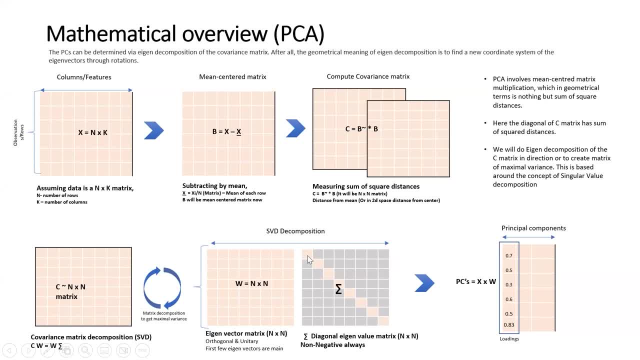 Now, eigenvalues is nothing. when you, if you multiply to Matrix with its transpose, you will always realize that diagonal always represents the sum of squared distances. Now, the sum of squared distance is nothing but what we were trying to maximize in this particular approach. Also, whenever during this decomposition exercise, 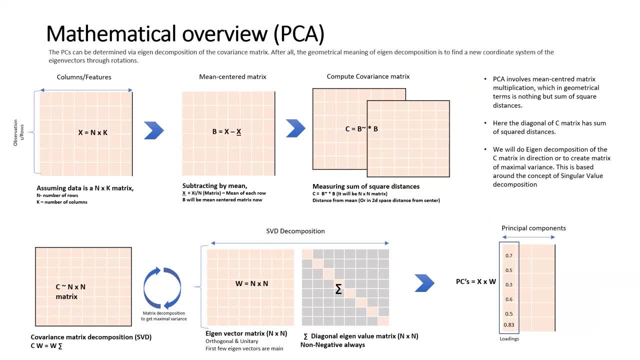 it's a rotate, iterable exercise And whenever a maxima is attained, that is when we say the Matrix has been completely single, decompose into its unitary Matrix, and there is the point when it stops. So that is when we can say that we have an eigenvector Matrix out. 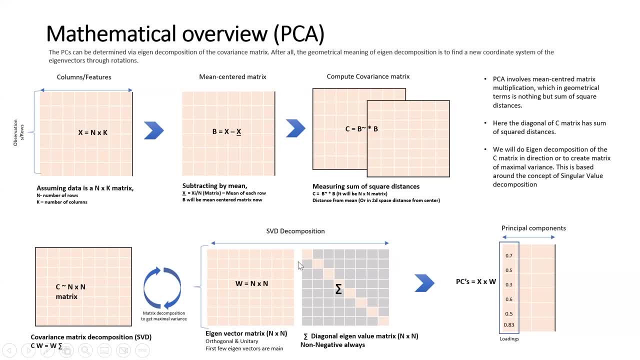 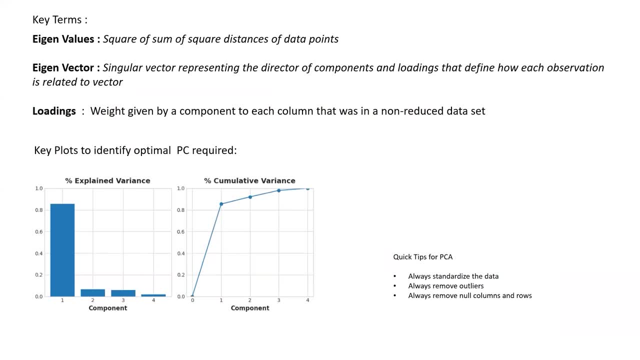 and using that, we can primarily create a principal components. Now the second aspects that come is: what is the right amount of components that we should pick in our data? What? where is the point where we should stop? So there's a before that. there's some key terms that I was mentioning in the previous slide. 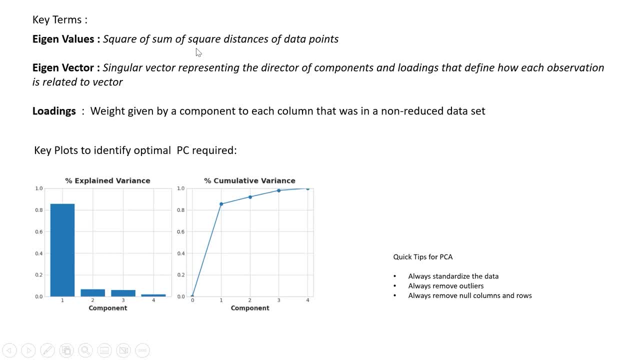 Now eigenvalues is nothing but the square of some distances of the data point. So, whatever data points we had in the original sense, what is their sum of squared distance from the origin or from the mean? So, either way, if you are, if you have standardized the data, 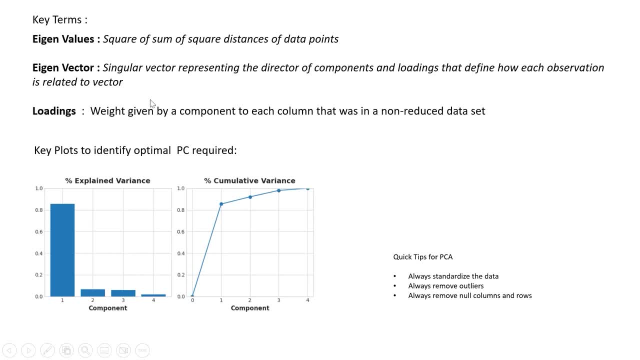 your meat will be zero. So that's why I was saying from the zero point. The eigenvector is a singular vector representing the direction, Also the loadings that is there. So let's say a particular vector represents four or five columns, the values within them. 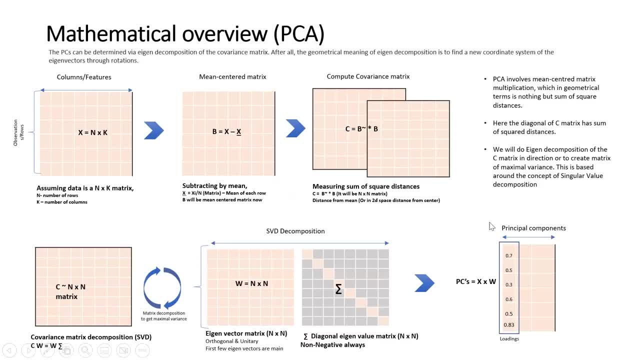 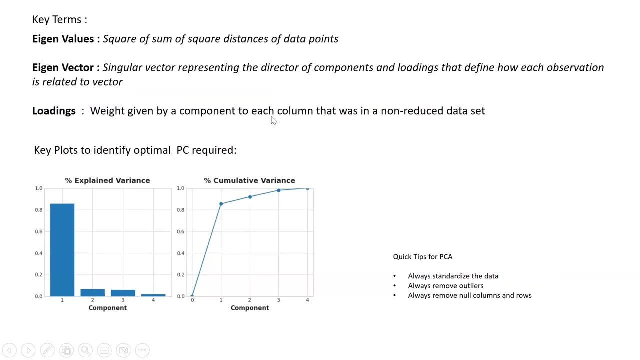 or the loadings within them, as I was showing in the previous slide. The values within them is basically: the losing is the weight that it gives you to each column. that was there in the data. So that's how we have to interpret what a vector is and the loading is, as I was mentioning, is the weight given by a component to each column. 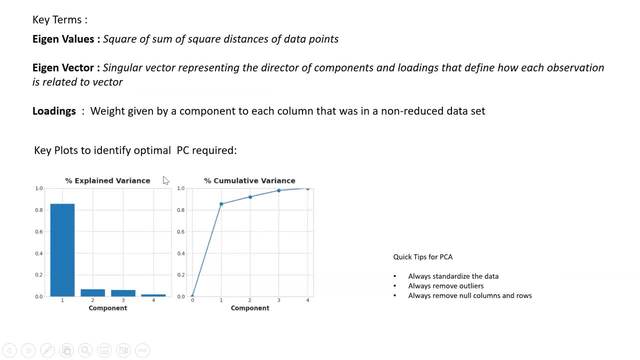 That was there in the non-reduced data set. the key plots. the one which I'm showing Right now is: this is called a scree plot, and you can even do a histogram plot as well- The whenever you are running PCA. you also need to understand the variance that the P component explains. 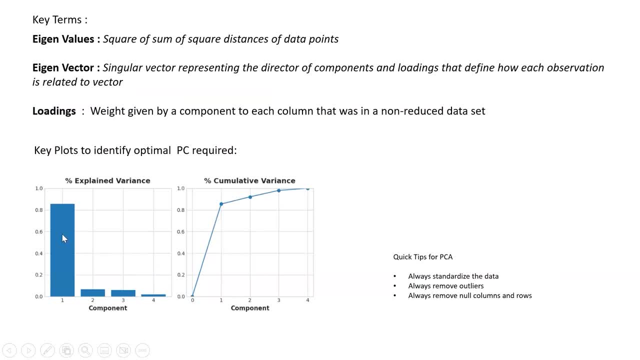 So if you do a covariance of PC1, it will give you some certain value: PC2, PC3. And if you feel like that 80 to 85% of variance is explained by your component one, then that is also sufficient for you to run your further analysis or a build, build a model top on of it. 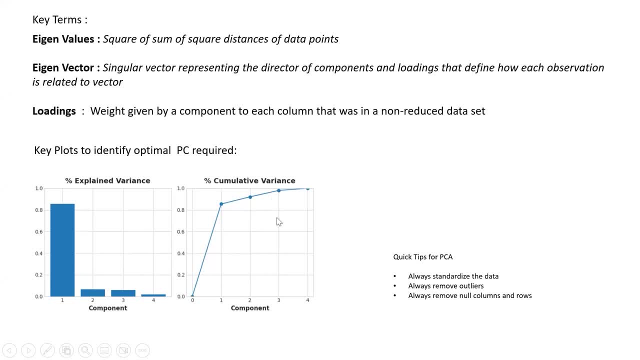 You can even build a cumulative variance plot which is nothing but a scree plot, and you can take it up to the level of hundred percent. but it is always advisable that you can keep up to two components or three components where, as and when, you are passing the 80% percent threshold for your components. 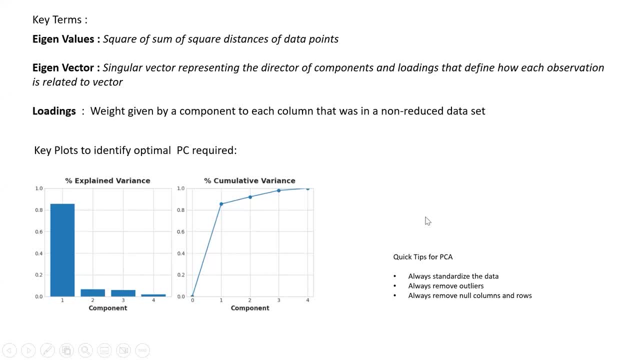 Few quick tips around PCA, as I will keep talking about it. You always have to standardize your data. There cannot be any null values across columns or rows when you're running this exercise And there has to be no outlier, because your component could be biased. 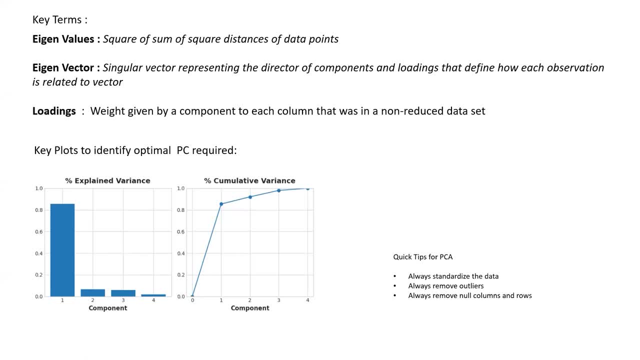 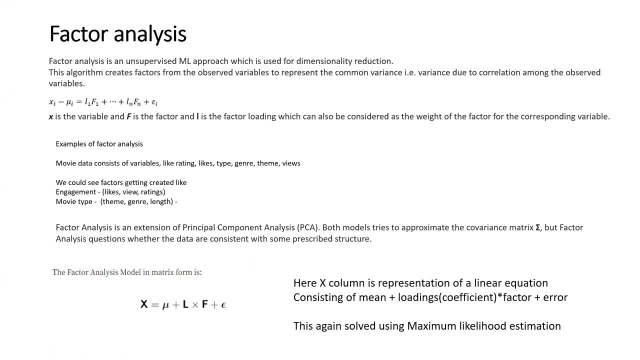 toward one of the data point, that is, skewing your data. So that is something that you need to always take care of while running this exercise. moving forward in factor analysis: It is nothing but an extension of PCA, only it is there. We were talking about matrix multiplication and how we decompose a matrix to get this out of it here. 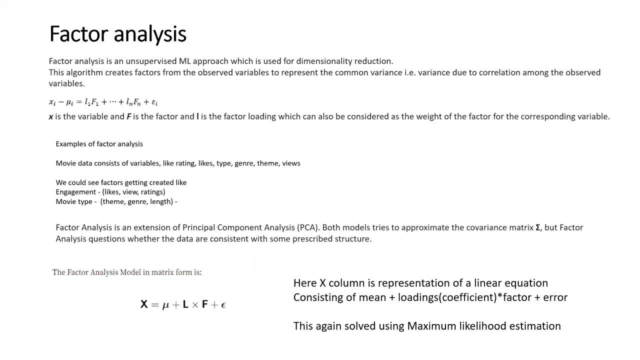 The approach is slightly simpler, but also it can also be solved through a matrix approach. You can assume a linear equation in your head and each data point or each column could be part of a linear equation. So if you, for an example, let's assume a movie data set that consists of columns like rating, likes, type, genre, theme, views, 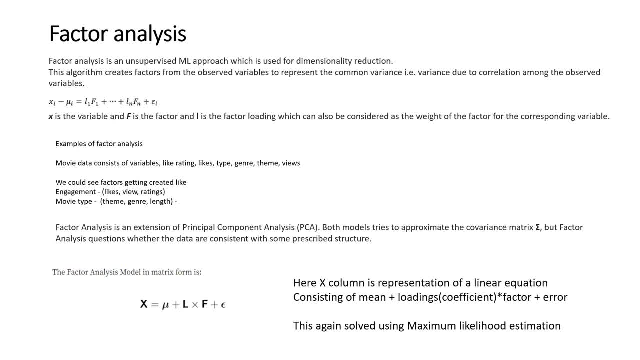 And if I have to, let's say, run a factor analysis of it, it would give me an output, something like it collaborates, feels like, likes, view and ratings, and I can interpret that as something called an engagement of that particular row or that particular movie. for this data points were there. 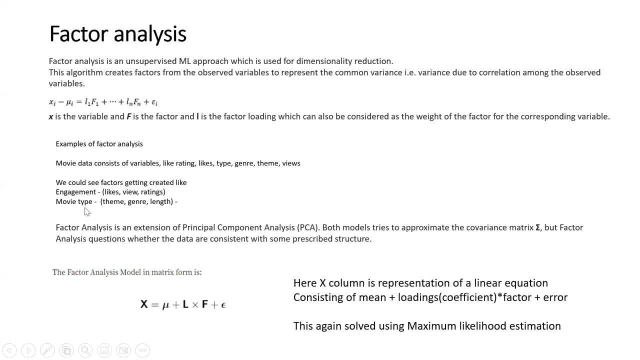 and theme, genre and length of the movie could be something related to movie characteristic or a movie type that were collaborated together with factor analysis. So with factor analysis, the approach, what we can interpret is we tend to collaborate or combine the variables that hint towards a similar thing. 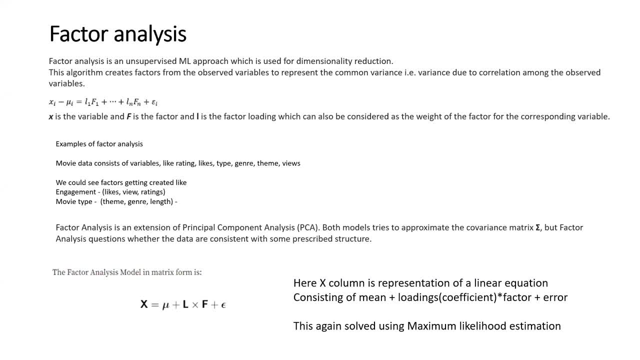 or a similar or are pointing towards a similar direction, And that is what it helps us in combining together. the how it does is: you can imagine, let's say you had a hundred columns in your data- You pick first five columns in the data, try to form a linear equation in the first approach. 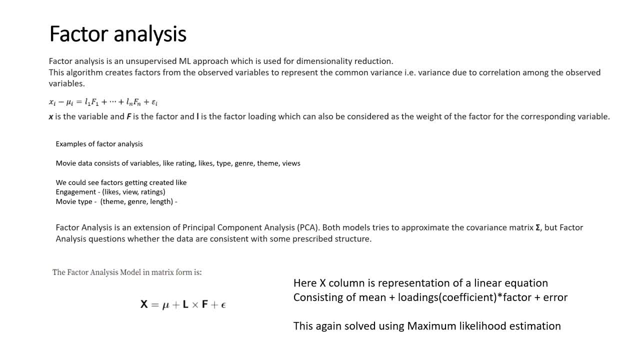 It won't be possible. But as you do the stepwise, the algorithm in factor analysis does this thing stepwise. So it picks the combination of variables, tries to see if there is a linear equation being able to fit, and how it does is is nothing but like a maximum likelihood approach. 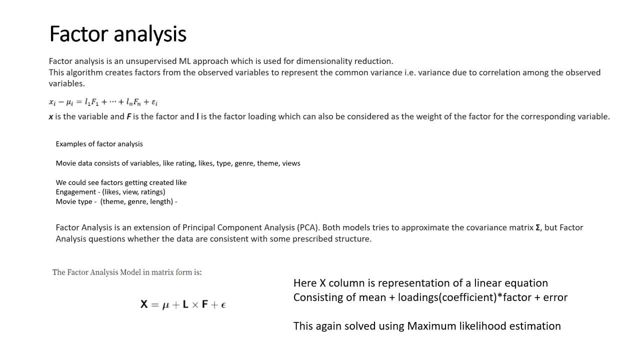 that we also use in our linear regression or logistic regression. They try to attain that minimum point where the error is Minimum and if, at that particular point, you are able to generate a particular factor out of it, That is what is the goal of this particular thing. 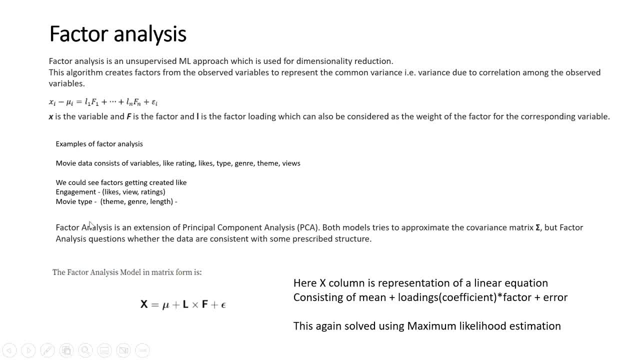 So again an extension of this, but again the differences in PCA, all the variables in the original data set were combined together to form a component one, or basically the component one had all the data points or all the information that was there in the initial set of variables in one component. 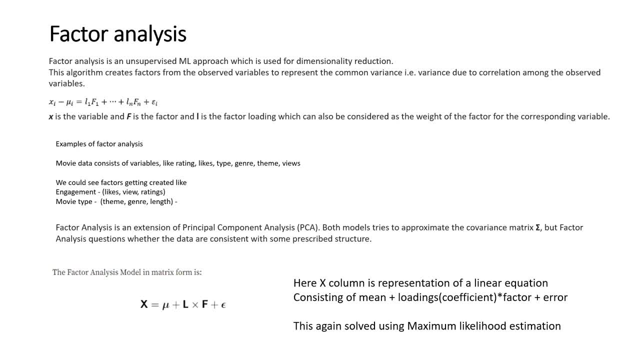 Whereas factors will not possess that fact. one factor Could possess only information related to two, three variables, where other factor could have for other three variables They are. when you are running a factor analysis, A good check is that your factors are not very correlated to each other. 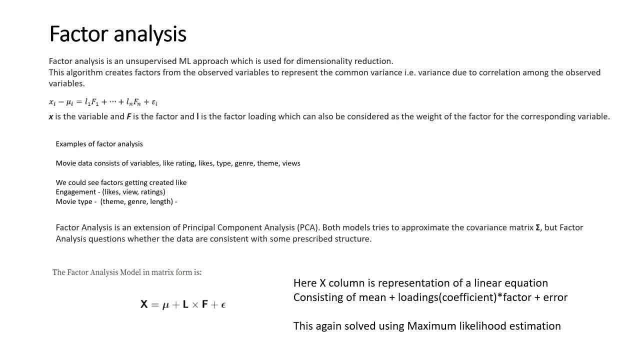 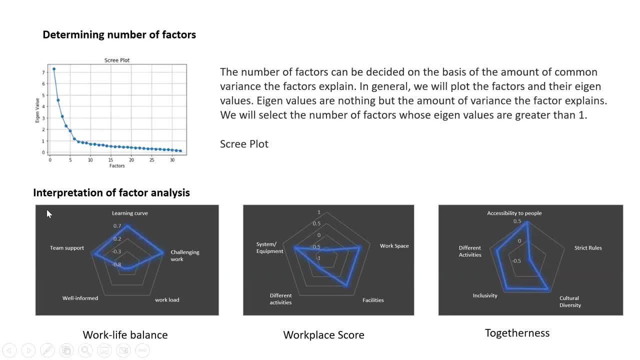 That is where, when you can say that all my factors are equally good, well created and they are exhaustive from each other, and that is the one check that you should always be doing. now again, just like how, there was a question in terms of determining the number of factors that are there. 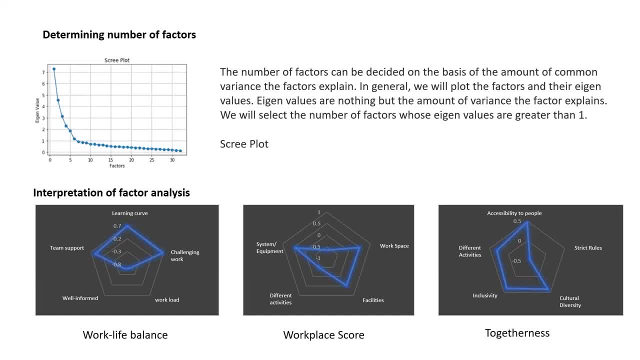 So, just like this is an inverse way of scree plot, but we are doing the same approach, even factor analysis will give you a gun values for all the factors that you create in your data. It will not be like that You have a factor created and you are not able to interpret it. 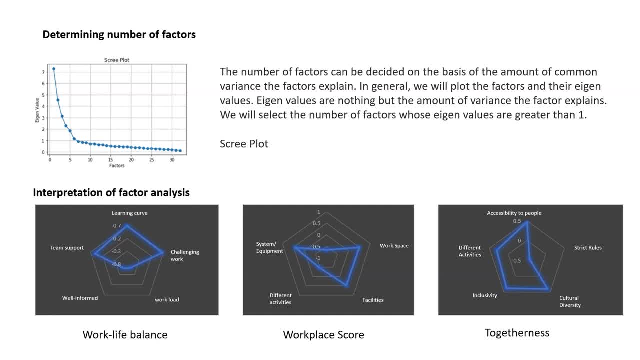 And how do you know what could be the cutoff fitted. So the best, or a thumb rule in factor analysis, or dimensionality reduction, like approaches like PC and factor analysis that always keep features That have a gun values greater than one, because they kind of possess the maximum information of your data. now 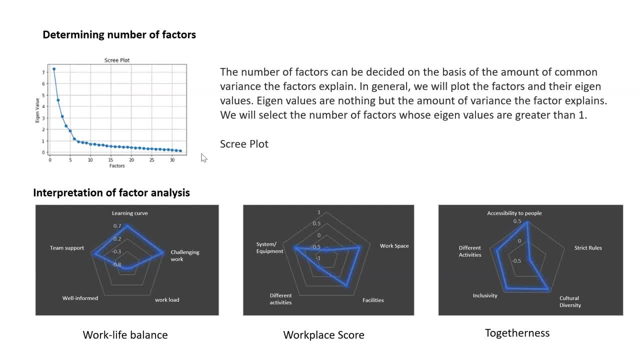 to walk you through a particular example of factor analysis here. I took a data set which was a kind of a survey data and kind of wanted to understand what kind of factors are created and whether I'm able to interpret this factors or not. So if you are not able to interpret a factor, 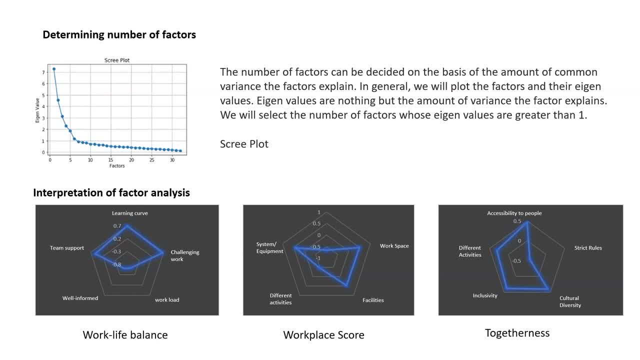 that means there has to be a redo of the exercise again, because usually factor analysis Give you a good interpretable format where we can make some sense out of what data points or what columns you have in your data, The. what you see here is a spider plot. 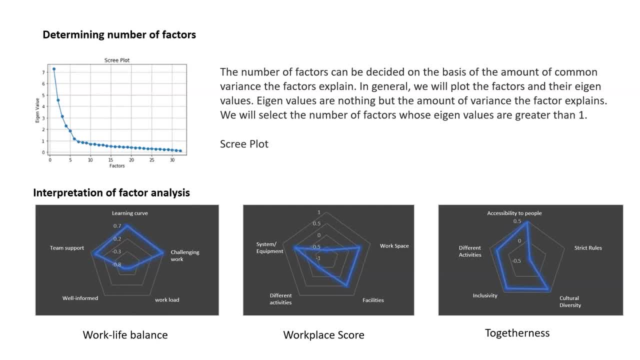 and that is one of the key plots that you can also use when you are working around factor analysis or cluster analysis. It gives you a good sense of understanding that particular cluster or factor or components. So it's a good visualization approach that you can consider while running these kind of exercises. 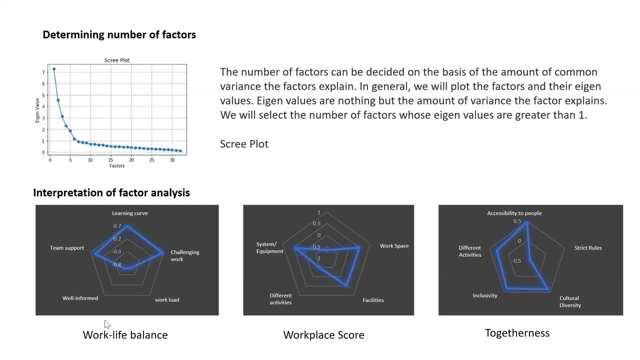 Now when talking about this particular survey data. so I had question. I related to different kind of formats and we all had to like in that particular survey, Everyone had to give a certain kind of score to each kind of metric. So based on the responses that were there in the survey, 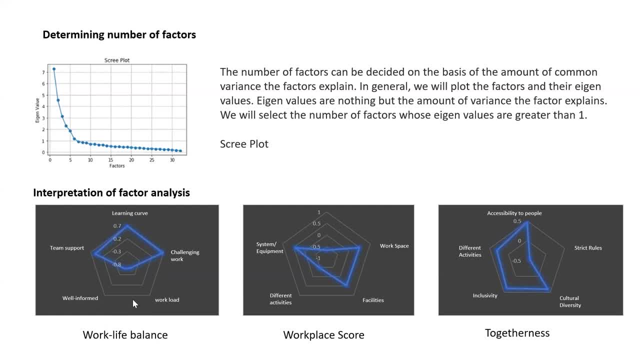 I kind of tried to run factor analysis to do it So once few set of variables that were. there is workload score channel, whether the work is challenging or not. learning curve in the workspace, whether they seem support or not, and whether you are well informed about your work. 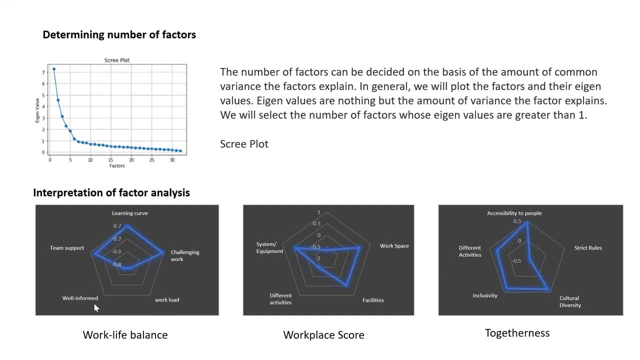 Now, if you can see, this is this was one of the factor created out of it, and it grouped five variables for, obviously, the key variable out of it was learning curve, challenging work and team support. So these were the three key variables that were driving this factor. 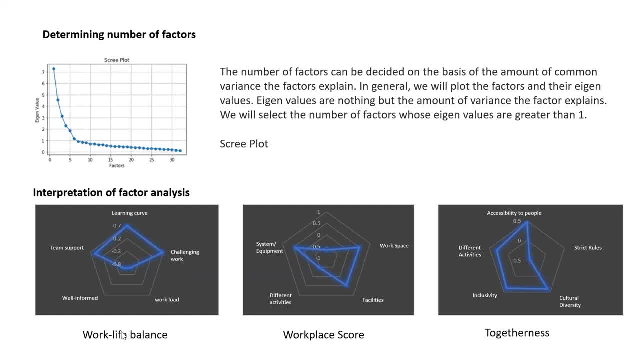 So that's why I named it, probably as something related to work-life balance. You are able to see team support, the work is not challenging, So something that hints towards a work-life balance. So that's how I will interpret this particular factor in the data. 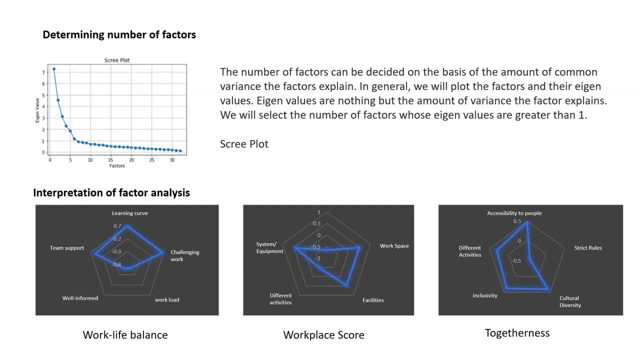 And whenever you are running a visualization or explaining it to your clients. Also, it is a good way of showing and understanding that particular factor. Then again, there was some set of features in the data that cater to. probably wanted to understand how's the workspace. 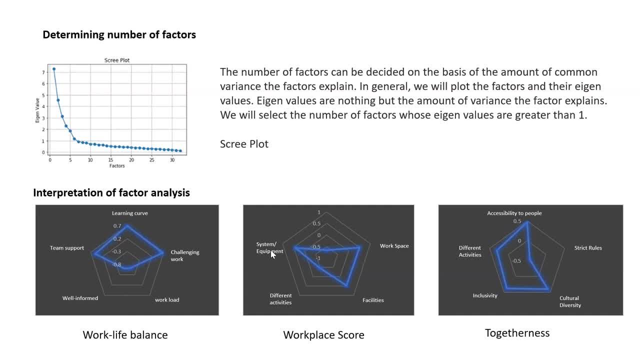 What kind of facilities are there? Are there any different activities, system and equipment. So it was only related to four attributes and you can see- I probably called it into the very layman term- as probably a workplace score, that how a person sees his workplace, and that's how the factor also, or the algorithm also, understand. 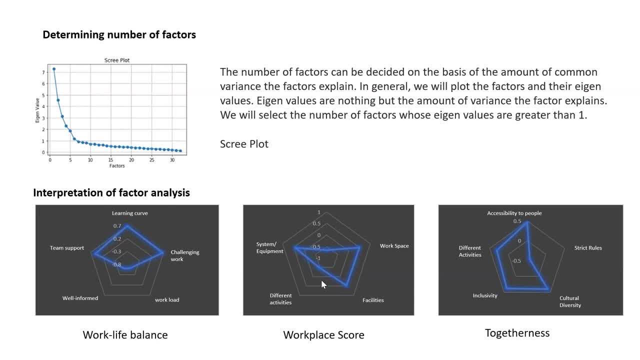 that these kind of variable should be clubbed together, because what you could see? that they, these variables, kind of follow a same direction. They might be correlated to each other, but not at a scale that we can drop one of them, but the direction in which they point, or the where they are hinting, the entire algorithm is the same direction. 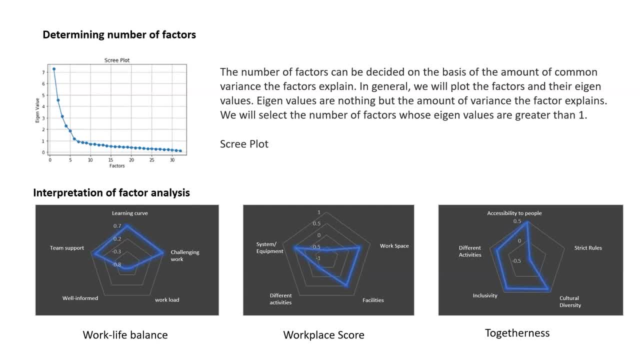 And actually, when you fit a linear equation, it tends to attain a Maxima as well. So that's why we see these kind of variables are grouped together as well. But there were other aspects to this particular survey, where it asked about cultural diversity and workplace. 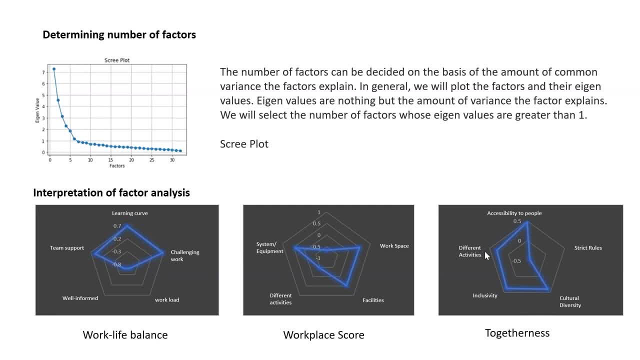 whether there are strict rules or not, accessibility to people, different activities again it's, and you can see there This is one use case where the variables are not exhausted, but we usually see they are mostly exhaustive and do not Overlap. here The importance of different activities is come. 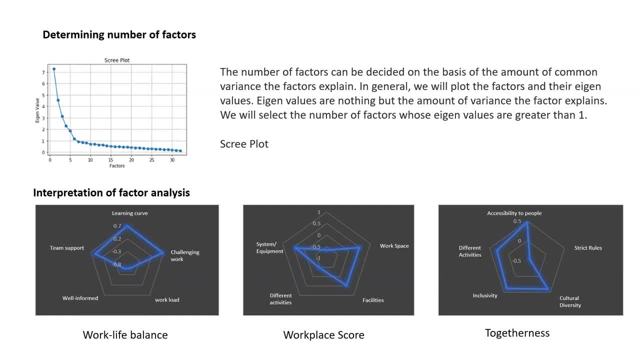 Whereas in this particular case we see that it is getting a higher weight age towards it and then inclusivity. So we could see that it is pointing at good variables and it has a lower score towards strict rules, But all of them, these variable kind of point at the same direction. 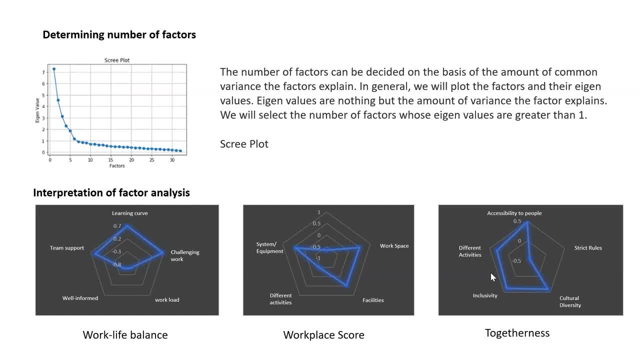 So cruel, like if a person is saying there is inclusivity- and there are, we are accessible to people, then you might feel there are less kind of strict rules, So that's why it has lens less. It's important, or that's how the model has interpreted it. 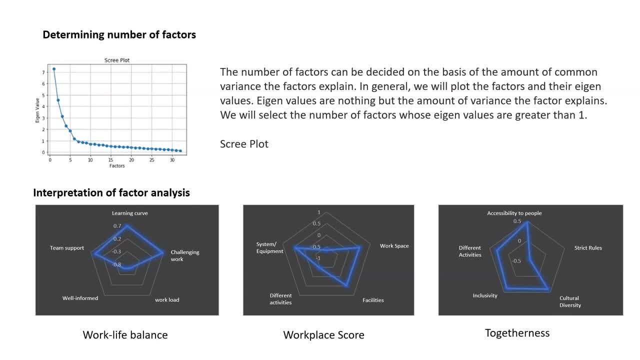 So this is one way of interpreting our factor analysis And this is one kind of a visualization approach that you can either use it- PC as well, or any kind of cluster analysis that you tend to use, and it will give you a fair idea of how a factor looks like. when I talk about PCA for this kind of visualization. 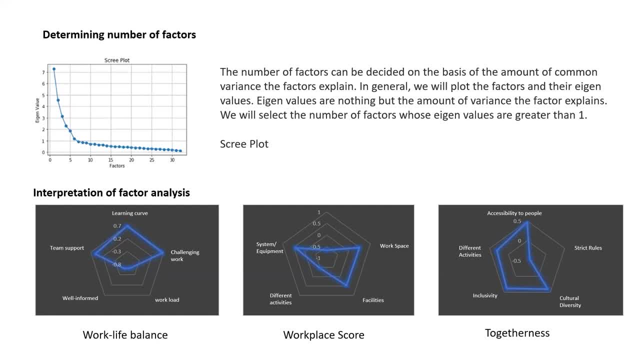 It might be very hard because it is made out of all the columns that are there. So then you will have to imagine a probably a spider plot of more than 10 edges where you have all these columns there and it is pointing out to someone. 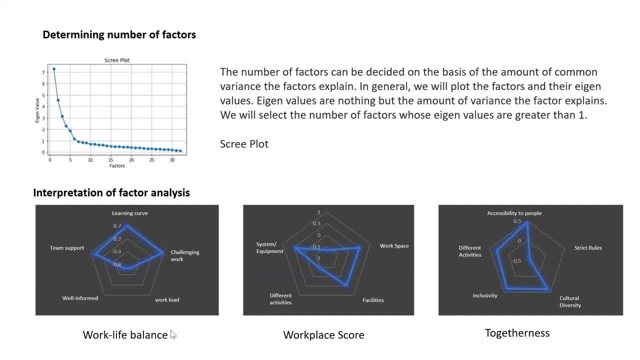 So then you cannot give it a name or you can tell that this component tells me this particular story only. So that kind of trade-off always exists when we are looking at this a particular thing. I'll probably take a pause and see if there are any questions. this question on. 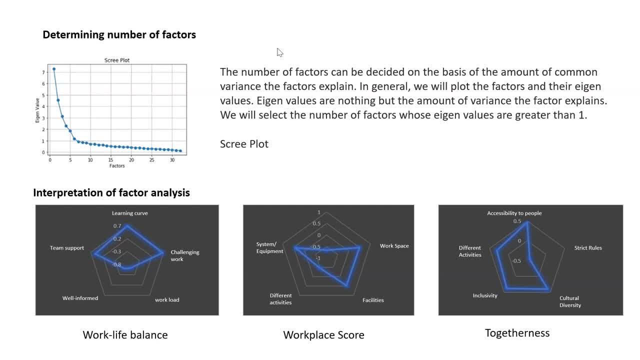 How to standardize the data. So, in terms of standardizing the data, we usually go by approach of subtracting each of your, so there are multiple approach: min-max scalar- I have spoken about it by last session, So there are multiple approach. 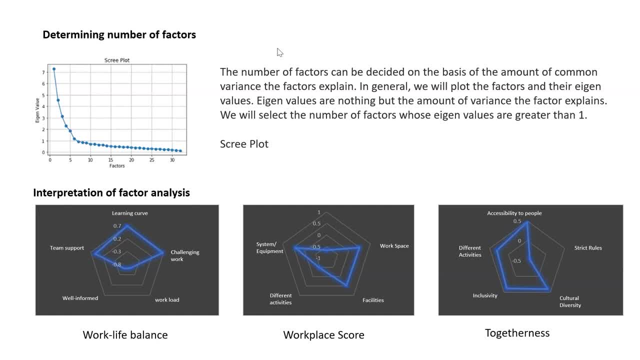 You can scale your data between minus 1 to 1 or 0 to 1.. But the basic funda around this is that you, for each data point, you subtract that with your mean and divided by the total Total value of the data. if you still feel the ranges is high, 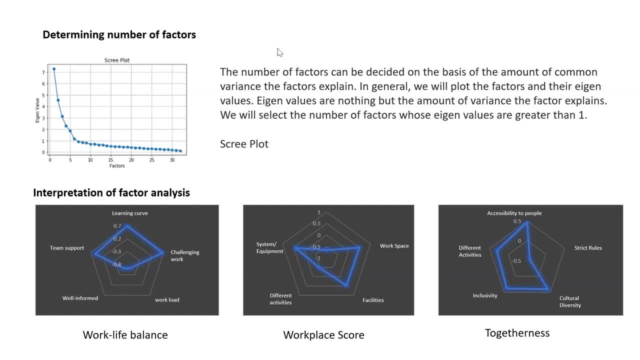 So this is the one, this basic way of standardization of data, data, data that we do in digital life. So there is no. the other question is around what number of features will require dimensionality reduction? So there is no size constraint to this particular thing. 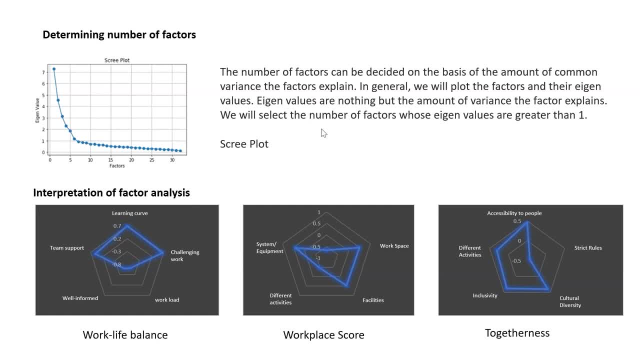 Whenever your dimension like, say you have more than three numerical three columns and more than ten, four or five rows in your data, That means your data is Already four cross five space. So that is something that you cannot visualize in a 2D plot. 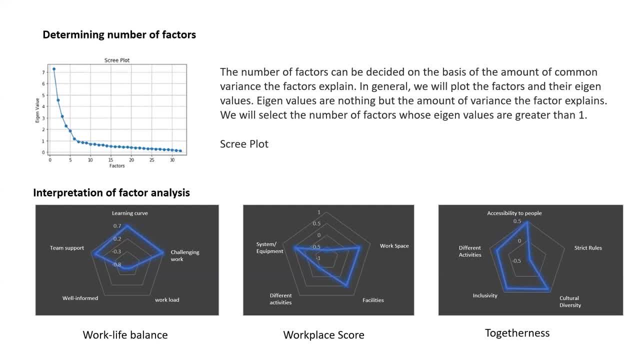 So the idea of PC or factor analysis, that you can visualize something in a 2D format. So whenever you go beyond that, there is always a scope of applying these techniques, but I would recommend that whenever you have more than 10, 12 variables. 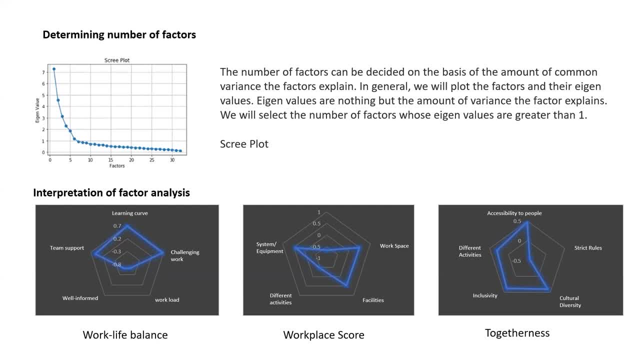 and you don't can't make much sense out of those variables, also in terms of what they interpret, what they infer. Then is the right time that that these kind of approaches should be applied on the data moving forward. I also have an example of PCN, and this is. this also ties back to the question. 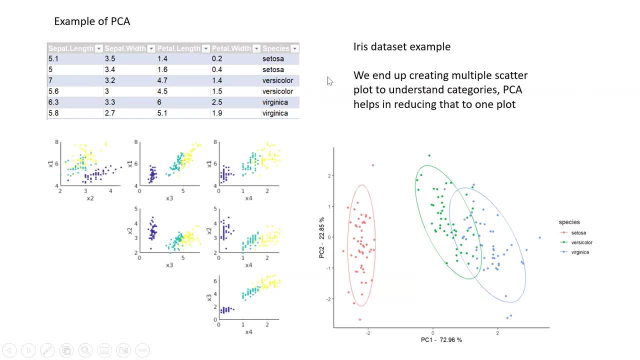 I was just answering. let's say, I'm taking a basic example of Iris data set, which is widely available everywhere, and I've just taken a snapshot out of it and you can see there are four numerical columns, one categorical column. Now, if I have to represent this column in a scatter plot and I cannot do it in one visualization, 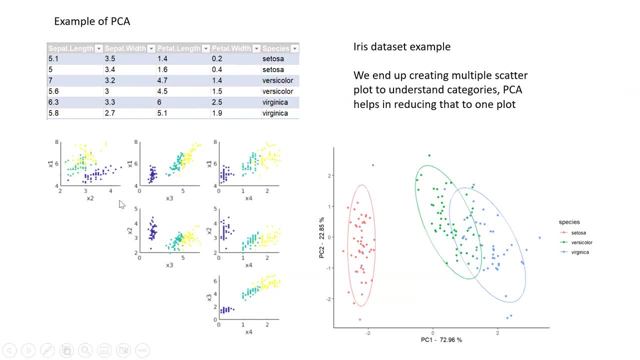 I'll have to create all these six visualize data that I've created. basically, it is divided by categories, differentiated by categories. I have one X is for one particular column, other X is for one particular column and the values represented in between is the third column. 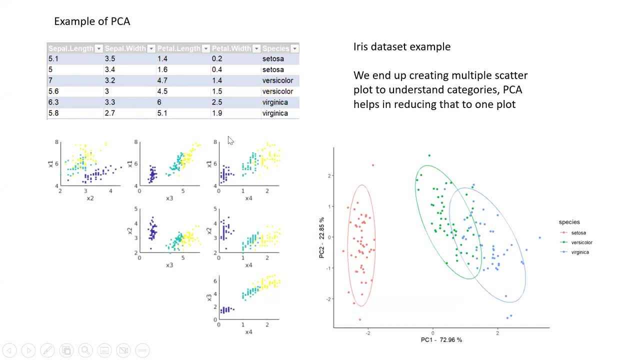 So I'll have to pay, probably create 3 cross 2 combination to basically see how these categories vary with each other. Now, if I end up running principal component analysis on top of that, I will be able to represent in a 2D format. 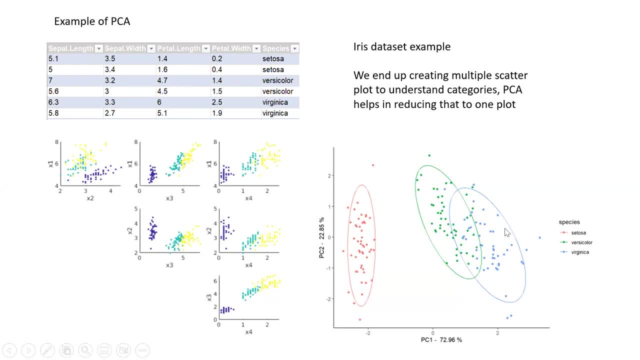 Now this is what. when I ran PC on this particular data, This is what I got. I could see clear clusters getting created out of it, and I could see both the components easily able to help me visualize how these three categories are related to each other, whether they are converging or not. 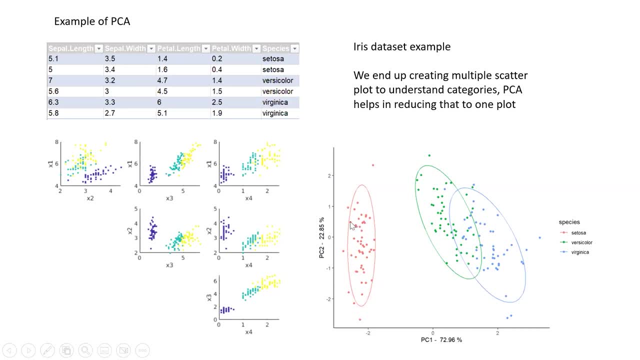 And if you imagine this for a huge set of data which has large set of columns in them, then it becomes a much better exercise. It is gives you a much better representation. This was a very small data and still that it is functional. 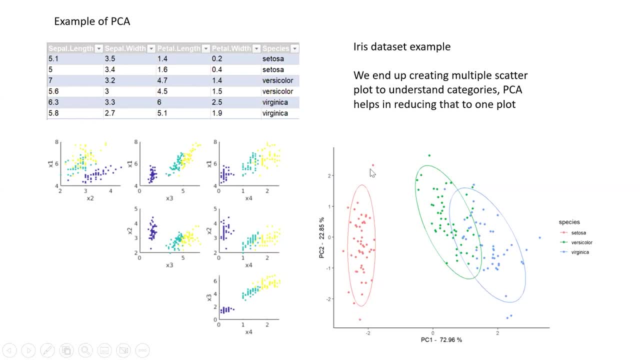 but the best use cases or the best practice of these kind of PCA analysis is when, when you run it on on a larger data set, Usually the best practices around or the best use cases are built around image processing use cases and textual data, where you have thousands of column. 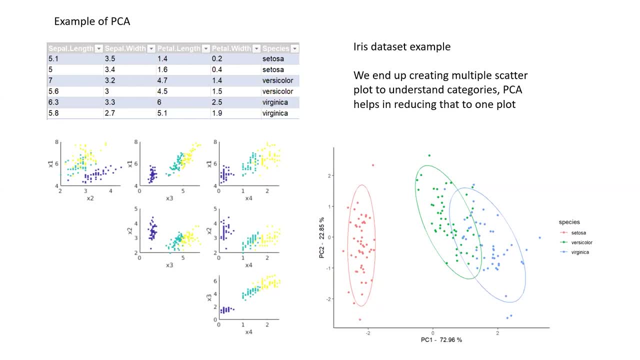 So whenever you resize an image into a numerical data format or you transform into a numerical data format- let's say you have RGB values, you have different pixel values at different different columns- that kind of data should always be compressed and it's a widely used practice that PS PCA is the best use case for transforming an image data or reducing an image data to data to two, three columns and then build a particular model on top of that. 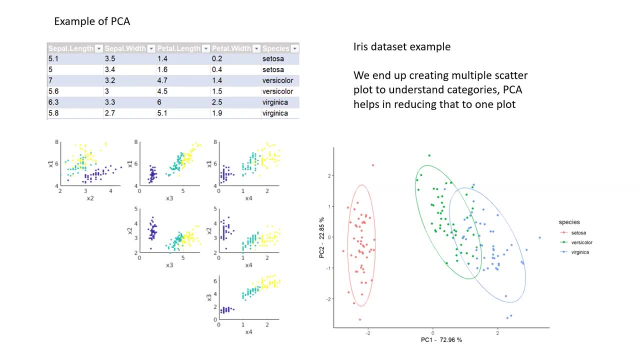 Similarly, when I talk about textual data, you have, let's say, a huge paragraph on which you create columns out of it. which the columns could be word at the values within them is the number of count of those words were present in that particular document. 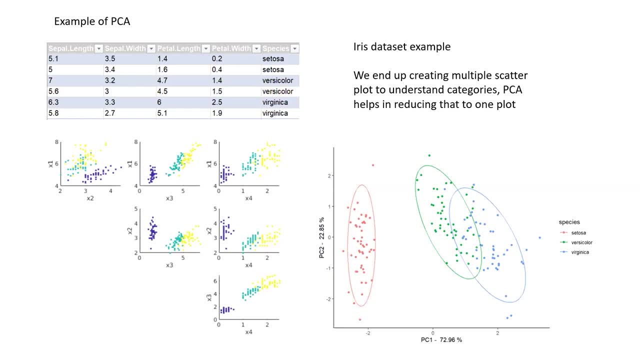 Now you cannot go through every word or n grams by grams that you create from the data, but you will have to concise that into a format that tells you the story of entire paragraph. So the one way of doing that is again PCA factor analysis. 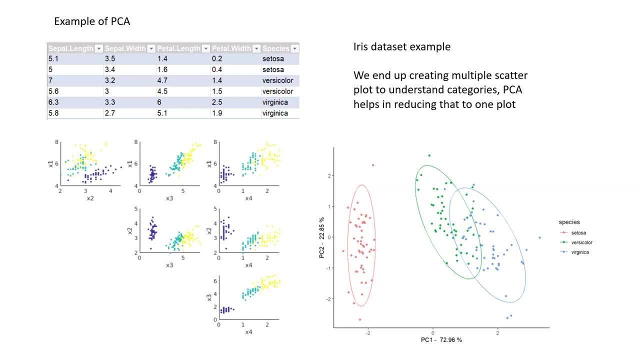 I also want to touch base something on the difference which is the best use case for factor analysis and which is the best use case for PC also. So when there is no issue around or there is no hunch around, explaining what your components are, 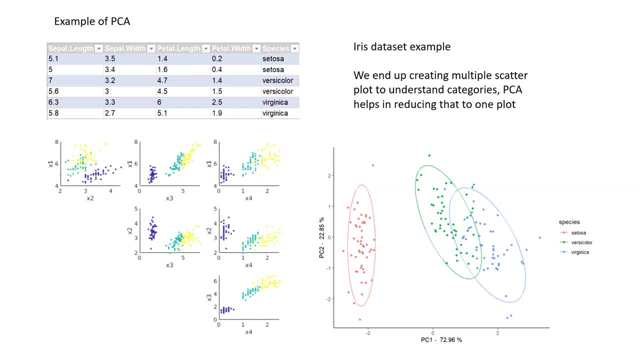 then it is always advisable that you go by PCA. and PCA is tend to be more sophisticated as is built on a more better mathematical covariance approach or a decomposition approach, Whereas factor analysis build on a linear equation. fitting of a linear equation. There now fact sometimes that there can be cases on this is one of the limitation of factor analysis that some of the various might not get captured in any of the columns or any of the factors that are getting created. 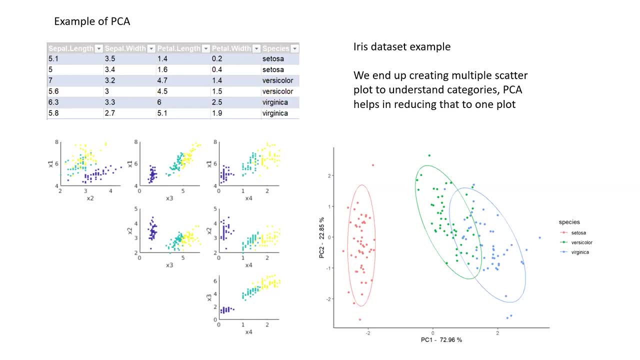 Now, that is, that is when that will happen. only with that particular column is interpreting or direct directing you towards a different kind of value only, or different kind of information from the rest of the data set. So whenever you have such kind of use cases, PCA is the best approach because it tends to take information from every column and put it in one component. 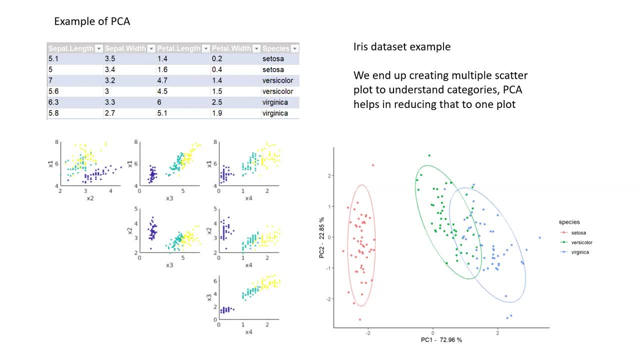 So, whenever you feel like you, there is no scope of you to reduce information, no scope of information loss, There is no scope of reducing your number of variables. You need the information with you. PC, I would say, is the better approach. There are factor analysis when you want to interpret. 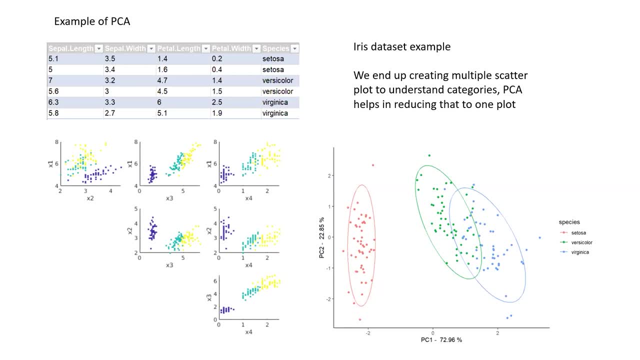 What are the combination or factor Getting created? that that is the approach that you should be looking at, though. So there is another question around PCA: considering a good values less than one. So no, we, both the cases We are considering a good values greater than one. 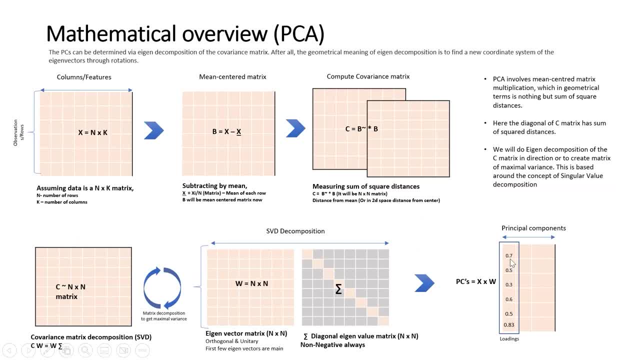 If you are getting confused with this, this is nothing but the loadings. So loading is the weight that a PCA component would give to each of the columns. So let's say there were K row K columns here, So you can imagine this as K rows now. 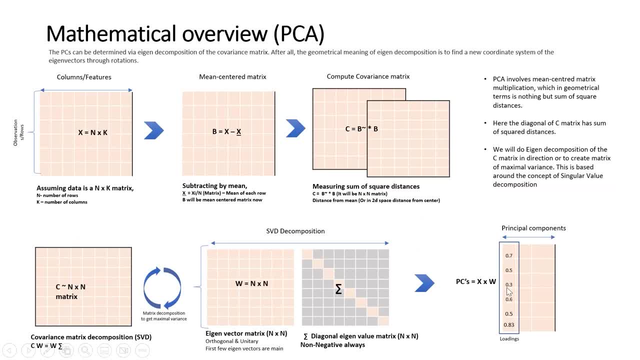 and this is the load That is associated to it. So for each of the column there there is a loading associated And if you go back and check the eigenvalues that the vector will be having, it will be greater than one for each of the columns. 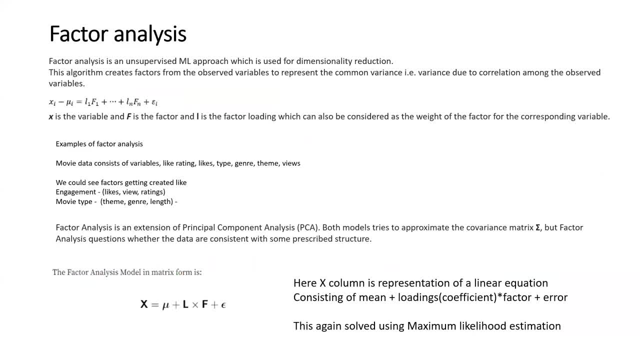 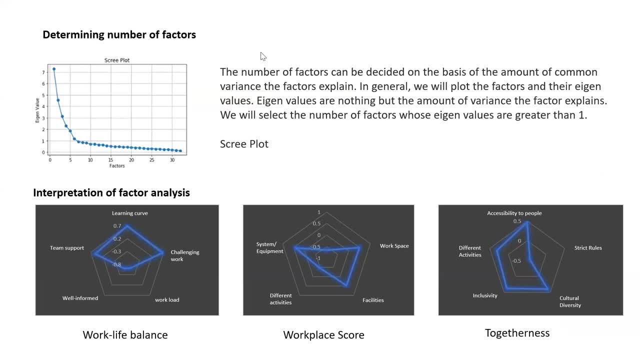 So that is always a thumb rule: Either you're using factor analysis or principal component analysis. Yeah, so image classification I was mentioning is the best use case for PCA. that you always have to go with an approach of dimensionality reduction there When you break down an image into a data set. 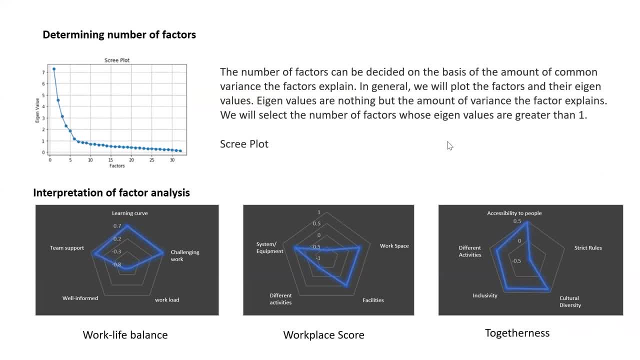 there are. the minimum column number of columns that I have seen getting created is around thousand 2000,. which captures for each pixel that is there, And if it's the images of a very high quality, then the column number of column also tend to increase. 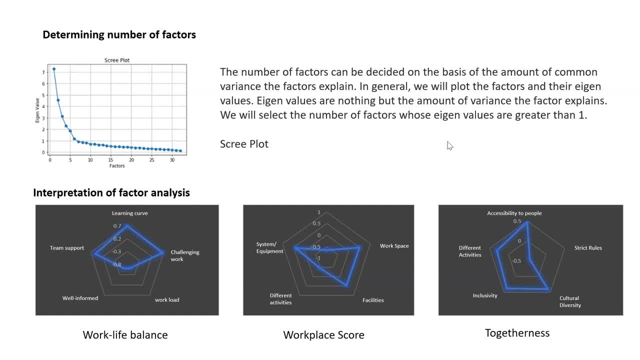 So their PCA works the best. It combines the pixels that tell you a particular information. It combines the pixel that, let's say, some color pixels of red Are combined together and you see that as a component out. Similarly, from factor analysis you can do the same thing. 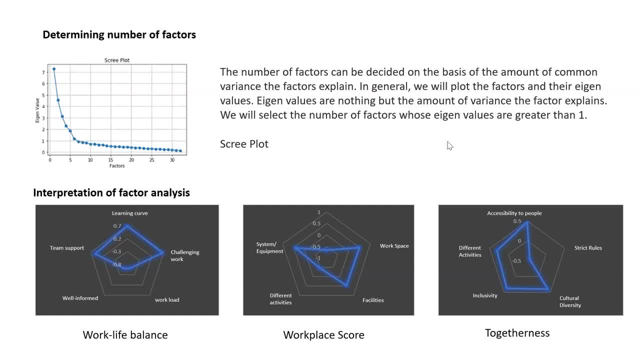 but PCA is again important there because you don't want to have any information loss Where, in factor analysis, dealing with an image classification data, you might tend to that the algorithm might tend to skip some columns that might not be fitting with any linear equation or part of any factor. 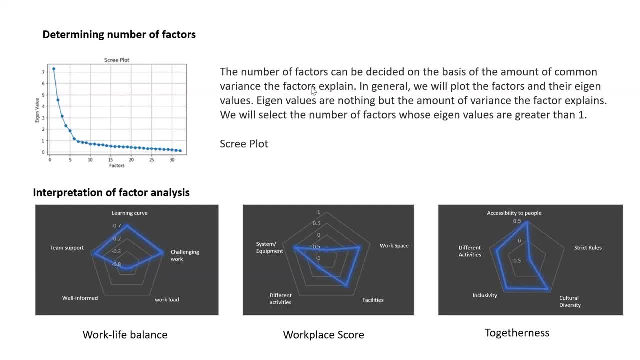 So, yeah, that's one good use case for PCA, For PCA there. If there are no questions further, I think we can close the session. That's was more or less on the PC and factor analysis. We'll be bringing forward few more topics around data. 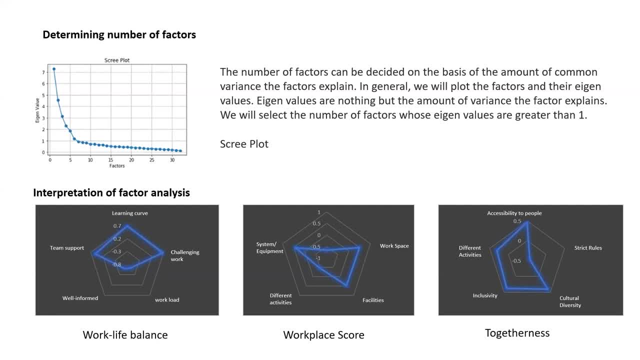 understanding how we transform data and then dwelling into the scope of how we enhance our models better. So PC and factor analysis is one of the two approaches. are the two approaches with which you can obviously enhance the performance of your models. It will reduce the computational time of your model as well. 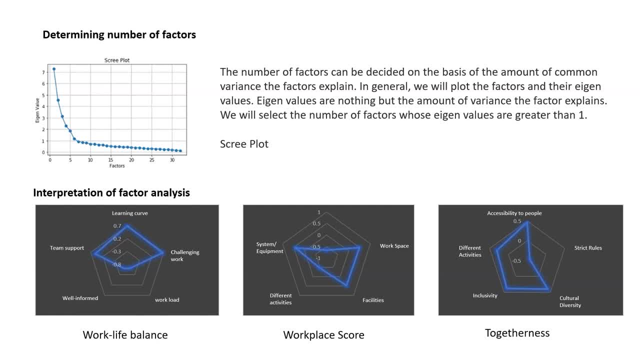 Okay, So there was certain questions on the chart as well. Let me go to them one by one. So dimensions are not same as column. dimension is the dot like the number of rows into number of columns. That would be dimension of your data. 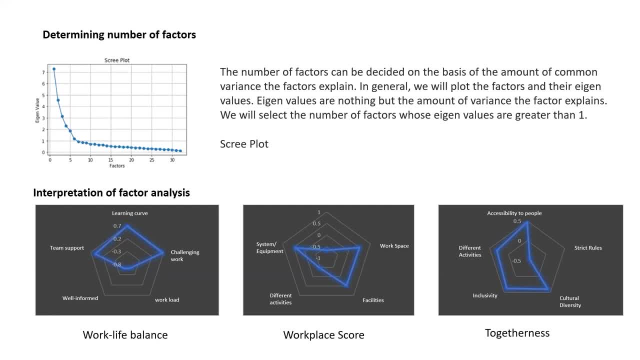 I have utilized ETS any, but again, it is based around a similar approach of clustering and the representation comes out similar to PC, and you will when you, when you compare these two algorithms, you won't see much difference between TSN E and PCA. TSN is obviously the more advanced approach of dealing with it. 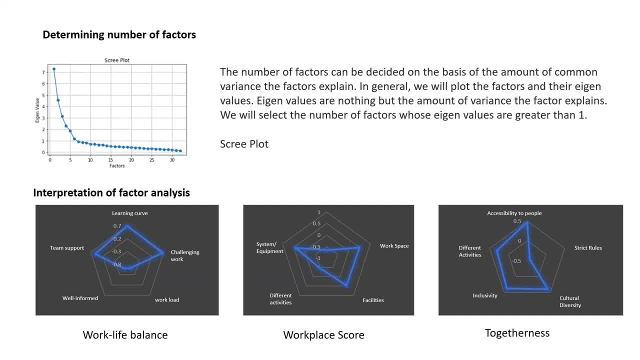 I think you answered this question of PC and factor analysis. Yeah, so you can. loadings, bait, weightage are all the same things which can help you like understand what a component is associated to. So if a component has, let's say you had K columns in your data set and there will be loading associated. 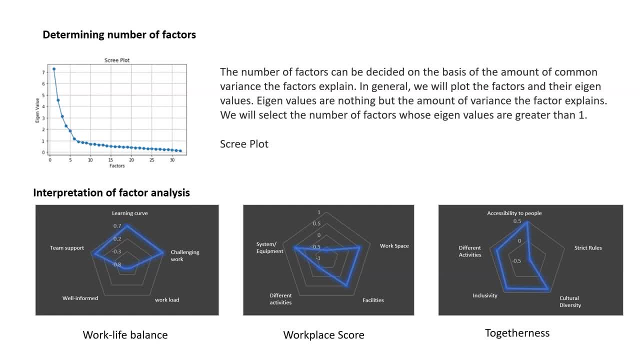 to each of these column with respect to a column. that will help you understand with the component is preferring which column the most. So, although it is a distributed paid that is given and you it's very hard to differentiate which column is has more waiting, but it's a good way to understand what your component or what your factor is made of. 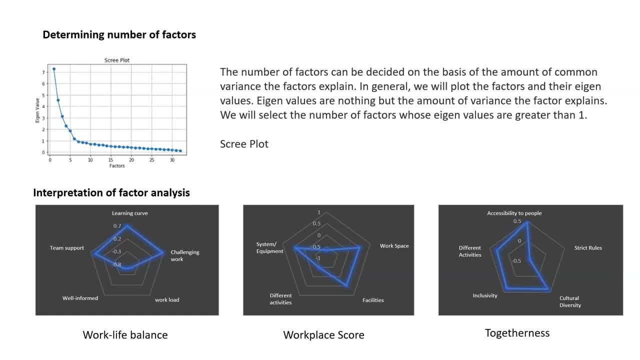 So that's why the weight is important. So the last question is: can we do clustering if data is having variables? So PCN, factor analysis, nothing but a clustering approach That you not apply row wise but column by. so that is the only difference. 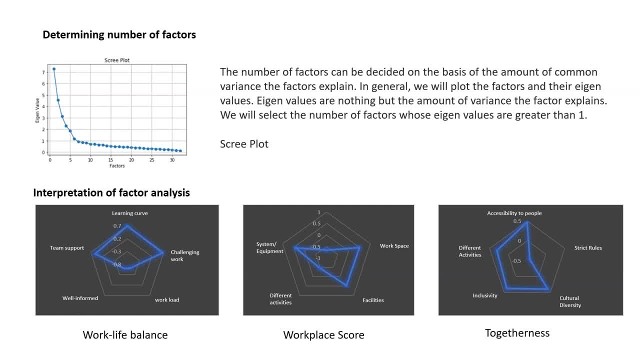 It's again an unsupervised way, like a means. Yes, Renuka, So that's. it's a similar way. It's an unsupervised way. as you might saw that, I was not talking about dependent variable at any stage. So, along with the deck material,